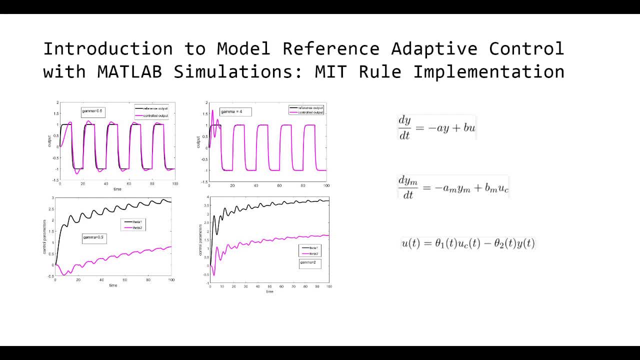 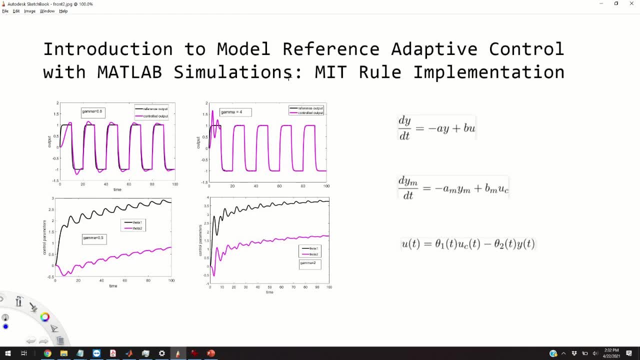 Hello everyone, in this video I will explain you the basics of Model Reference Adaptive Control and, moreover, I will explain you how to implement a simple Model Reference Adaptive Control algorithm in MATLAB. Everything that I will explain in this video can be generalized to more complex systems and to more complex Model Reference Adaptive Control algorithms. 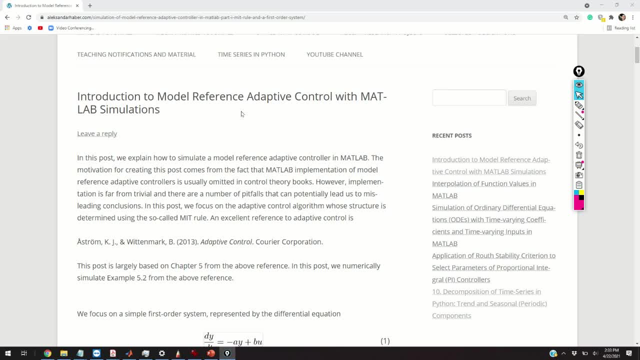 Ok, so let's start. This is the post I created that thoroughly explains the Model Reference Adaptive Control algorithm. But before I start, I need to explain why I created this video. Well, the motivation for creating this post comes from the fact that MATLAB implementation. 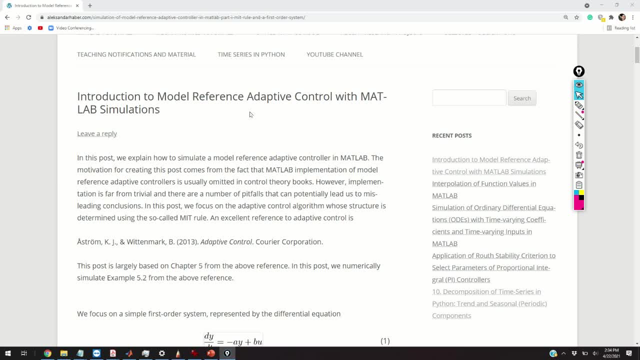 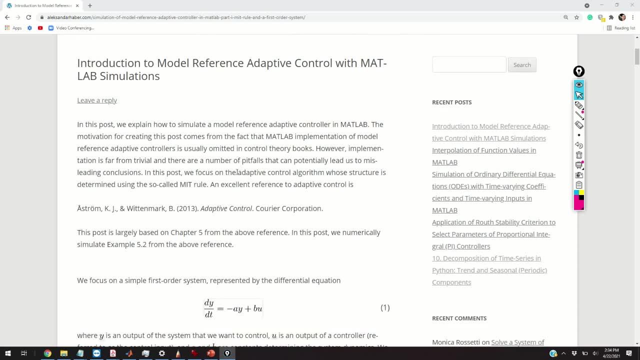 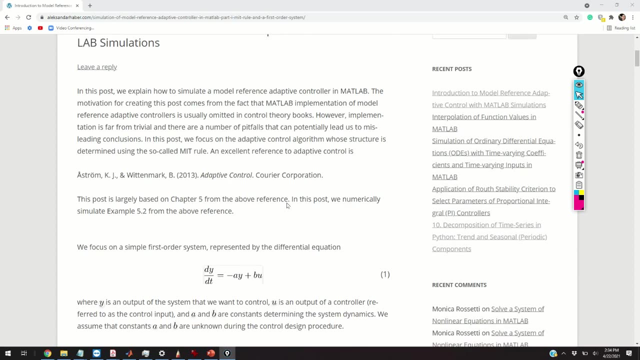 of Model Reference Adaptive Controllers is usually omitted in control theory books. However, implementation is far from trivial and there are a number of pitfalls that could potentially lead us to misleading conclusions. So, consequently, I wanted to clarify how to implement a Model Reference Adaptive Control. 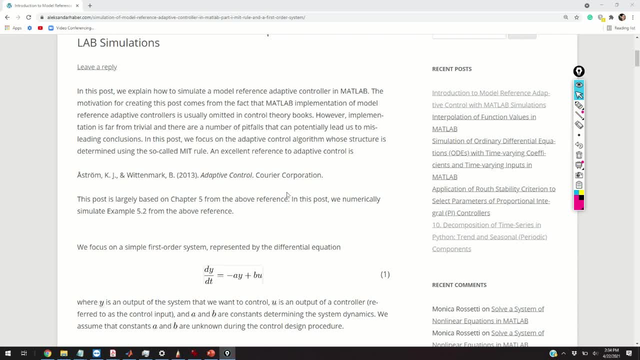 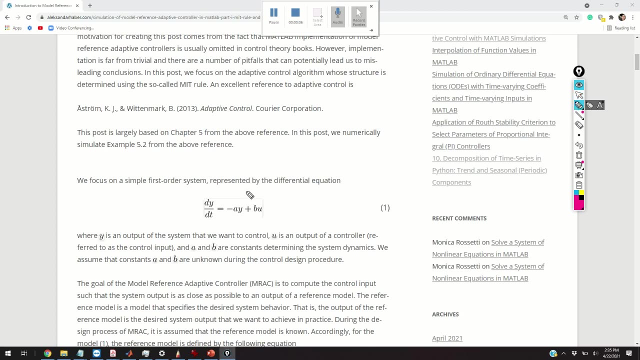 algorithm in MATLAB, since this is a very important topic that's often being overlooked by people who are teaching control theory. Ok, so let's start. We are basically focusing on a simple first order system represented by this differential equation. We have a plan that we want to control. Y is the output of the plan, A is the parameter. 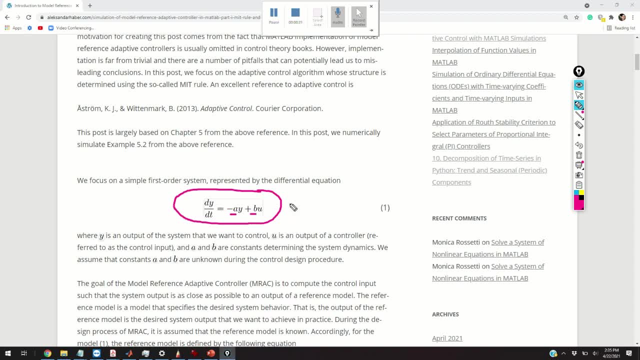 and B is the parameter, And we are assuming that we know the structure of this plan. We know that it can be approximated by a first order differential equation. However, we assume that we don't know the constants A and B. Now the goal of the Model Reference Adaptive. 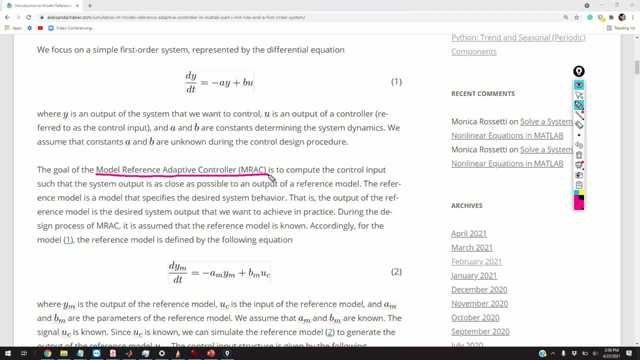 Controller MRAC is to compute the number of constants A and B. We compute a control input such that the system output is as close as possible to an output of a reference model. Now, what is a reference model? The reference model is the model that 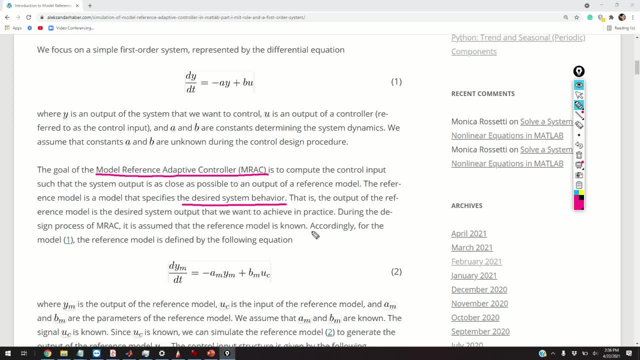 specifies the desired system behavior. That is, the output of the reference model, is the desired system output that we want to achieve in practice- And this is a general form of a reference or a desired system model, And we want our model, our plan, actually to behave in a similar way to the behavior. 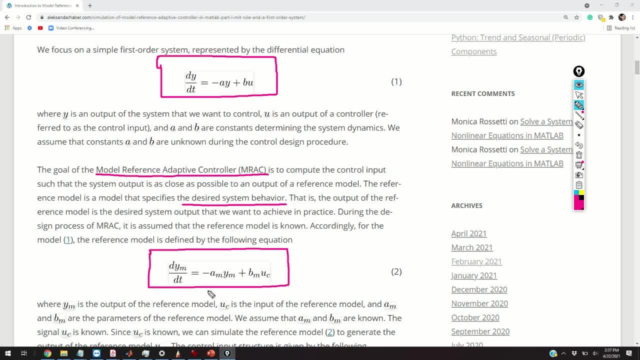 of our reference model, That is, we want this output, Ym, to be as close as possible to Y, Or the other way around: we want Y to be as close as possible to Ym And we want to find a control law: u as a function of y. 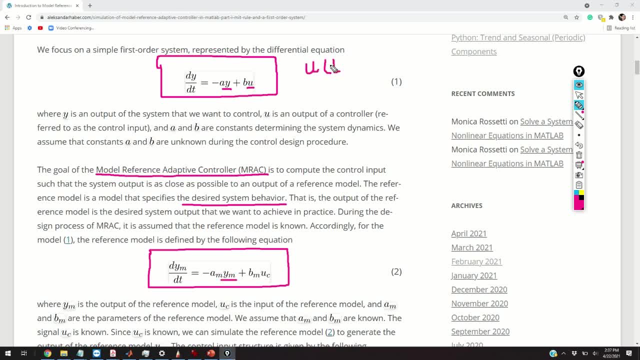 And we want to find a control law u as a function of y And we want to find a control law u as a function of y. Let us analyze the reference model. Let us analyze the reference that will couln meet three requirements we need to solve. 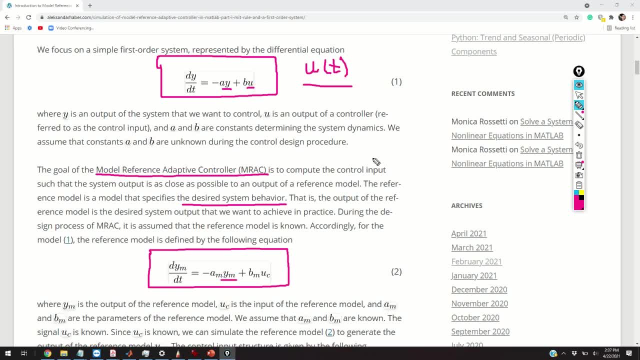 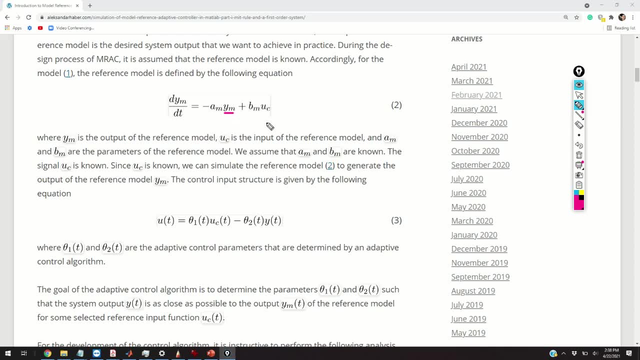 Let us analyze the reference model at the time that we will achieve that. let's analyze the reference model. Ym is the output of the reference method, AL is the input of the reference model and AM and BM are the model parameters that are. 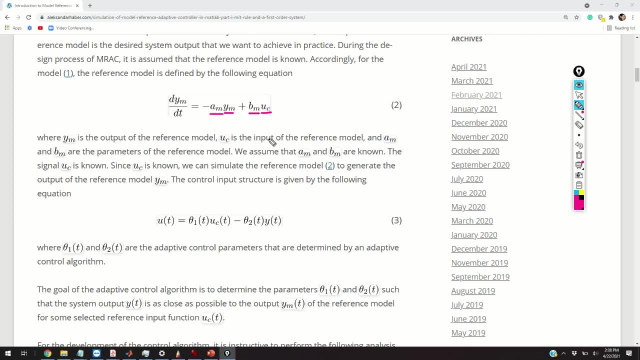 known. Since this is our reference model that specifies the desired system behavior, we assume that we know these parameters Because we use a model that specifies the desired system behavior designed them. Now, the signal UC is known. It can be a step signal, it can be a pulse. 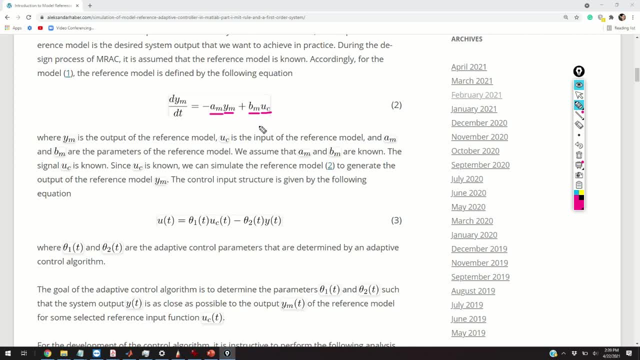 train, it can be a sinusoidal signal. Now, since UC is known, we can simulate the reference model, basically solve this ordinary differential equation to compute Ym as a function of time. So Ym is known also And we want to. 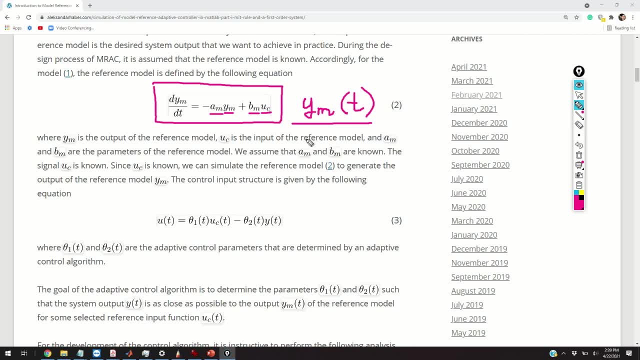 make sure that our plant or its output Y follows this signal. Now the control input structure that achieves this has the following form: We see that the controller itself takes the input to the reference model. it takes the output from the plant. so this is the feedback mechanism. so the control signal takes: 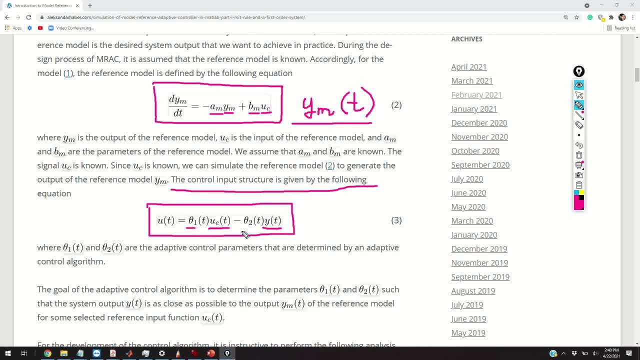 the output from the plant. and these parameters- θ1 and θ2- are the parameters that we want to design. So we want to specify these parameters. we want to find these functions- θ1 and θ2- as functions of time. So we want to find θ1 as a function of time and θ2 as a 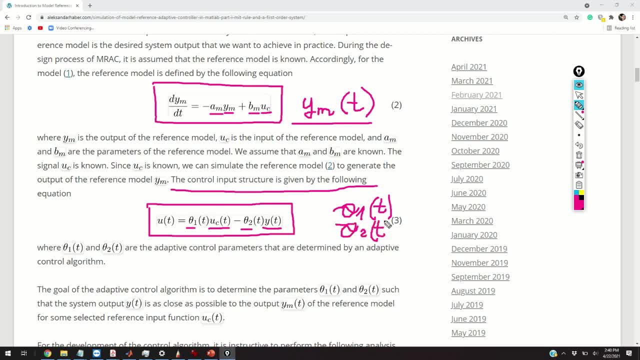 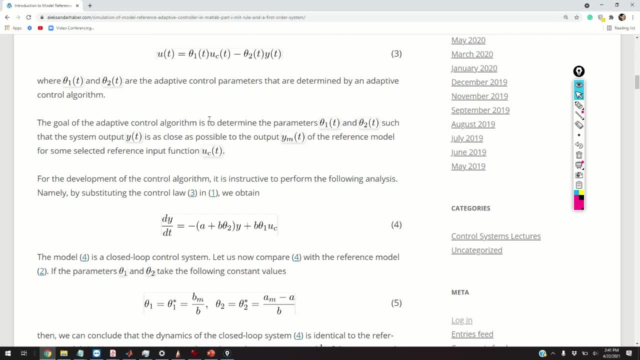 function of time. Let us summarize the control objective once more. The goal of the adaptive control algorithm is to determine the parameters θ1 of time and θ2 of time such that the system output Y is as close as possible to the output of the reference model Ym for some selected reference input function. 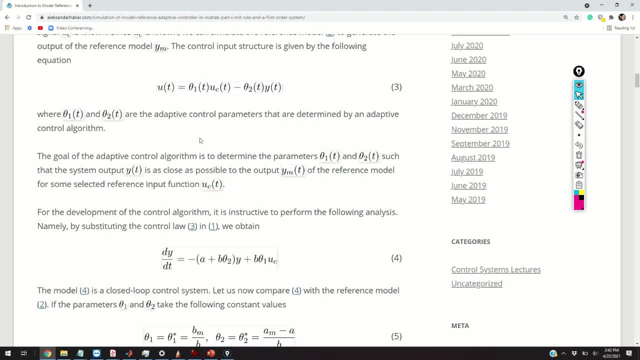 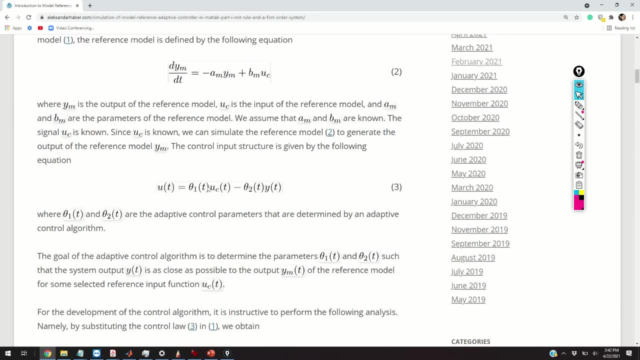 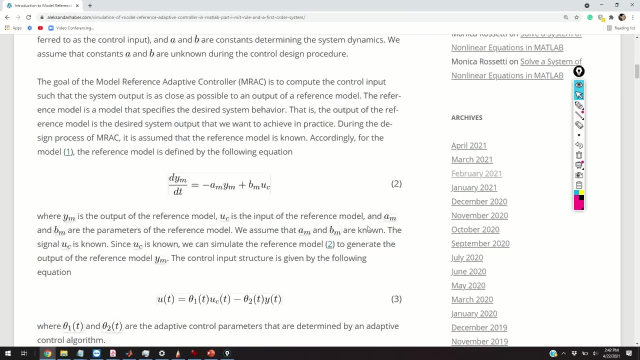 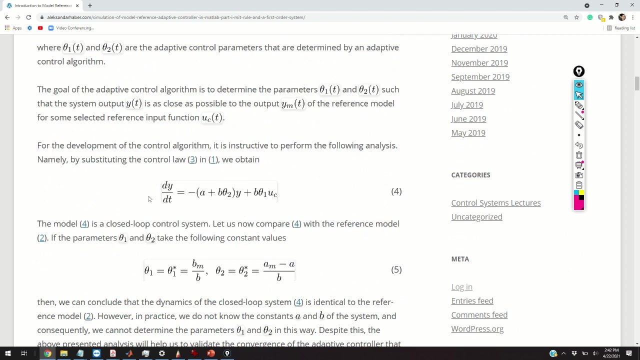 UC. So let us see how to achieve this control objective. Well, the first step that you need to take is to substitute this control algorithm in the system dynamics. So if we substitute the equation 3 in the equation 1,, at the end we will obtain the closed-loop system 4.. Now let 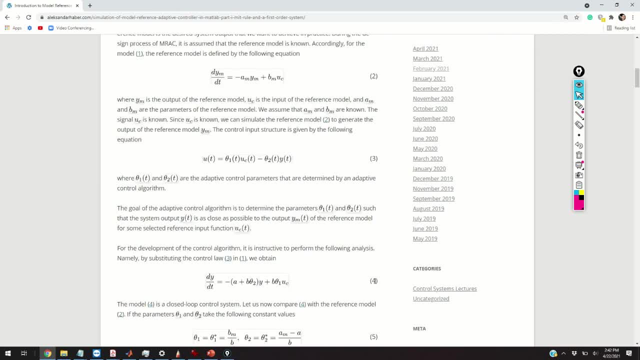 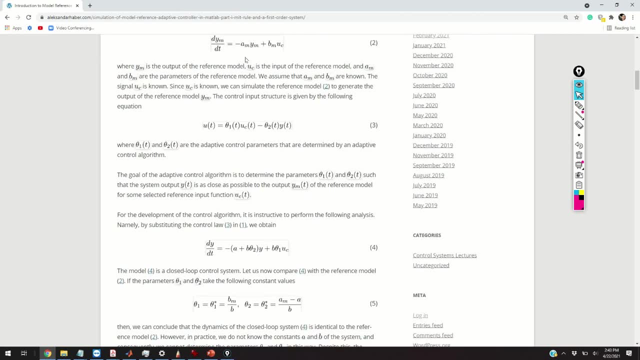 us analyze and compare the closed-loop system 4 with the equation 2 that specifies our reference model. What do we see here? immediately, We see that if our θ2 and θ1 are selected as the forms given in equation 5, we will see: 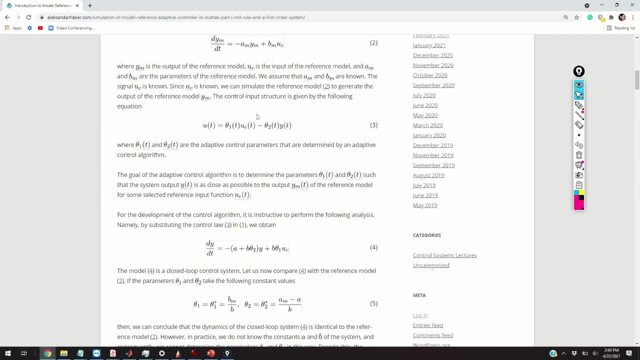 that, basically, this term over here becomes Am and this term over here becomes Bm. That is, we achieve the desired system behavior. However, the catch here is that we cannot determine the parameters θ1 and θ2 in this way, since we don't know a priori. 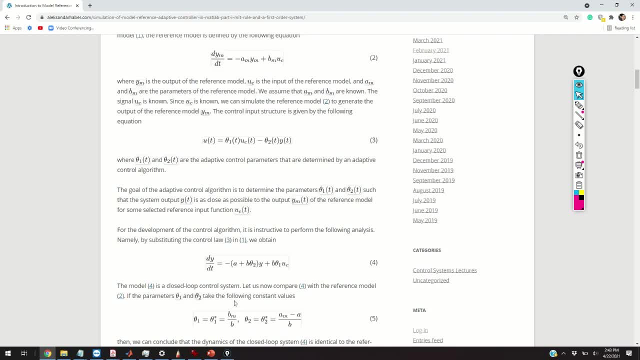 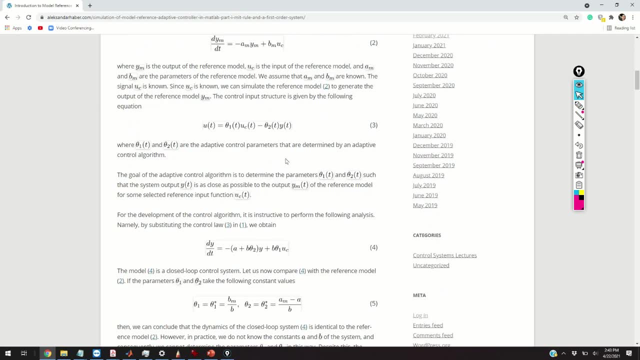 the system parameters A and B right. The plan parameters are unknown. The plan dynamics is unknown. We only know the structure of the plan dynamics. Nevertheless, the values of the parameters θ1 and θ2 that achieve the most optimal system behavior are: 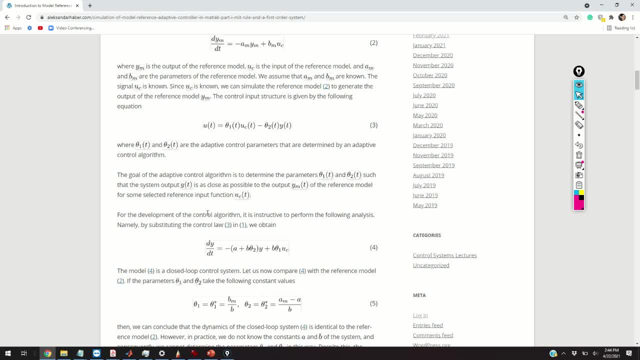 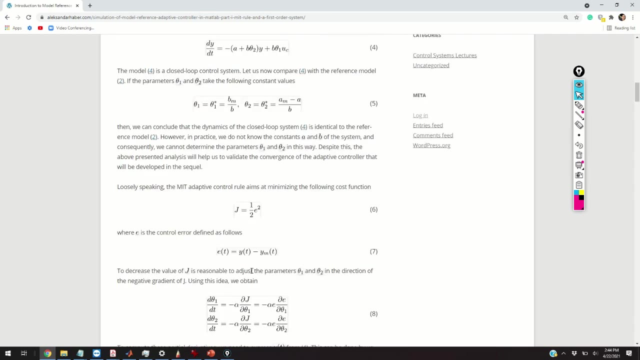 important for us, since we can verify our simulation results If our control algorithm is designed in a proper way. our parameters θ1 and θ2 should converge to these values in our simulations. Okay, Now the next step is to derive the algorithm. So there are many. 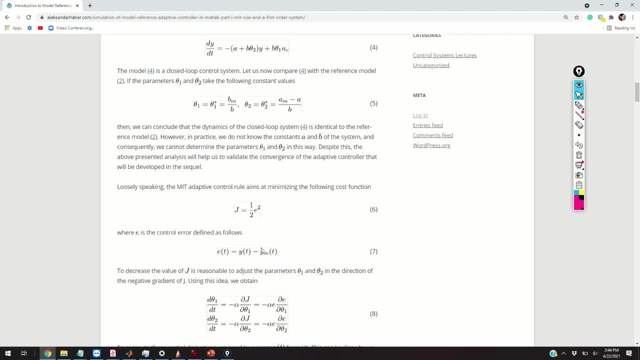 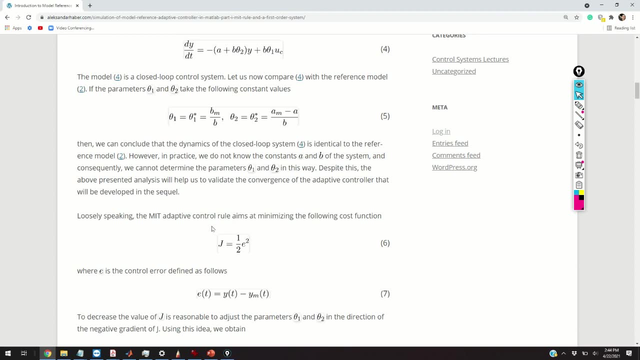 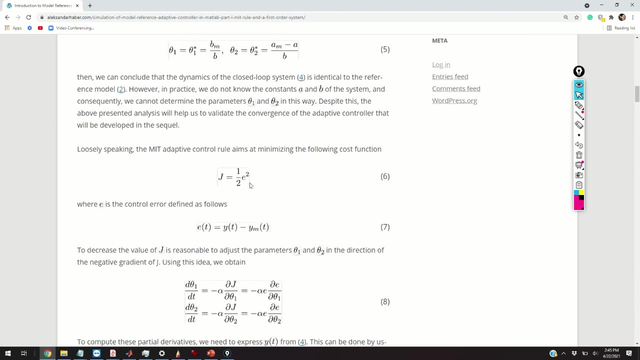 ways of deriving the adaptive control algorithm. We are going to use the so-called MIT rule. So what is an MIT rule? Loosely speaking, the MIT adaptive control rule aims at minimizing the following cost function. So we take the error, we square the error and we are trying. 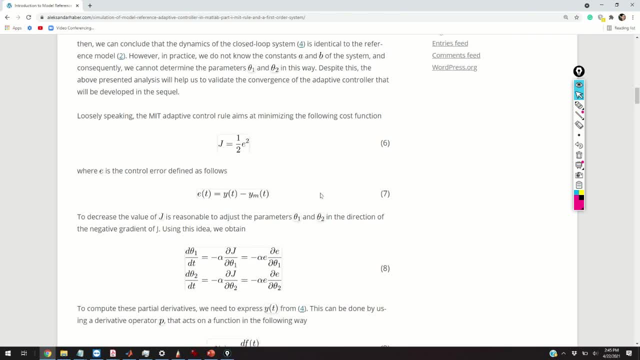 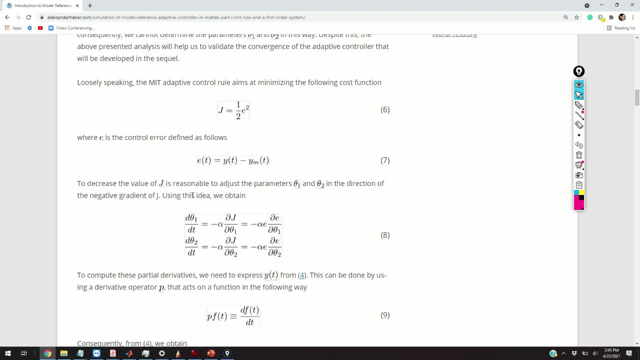 to minimize this cost function where the error is simply the difference between the output of the plant and the output of our reference model. Now, to decrease the value of j of our cost function, it's reasonable to adjust the parameters θ1 and θ2 in the direction. 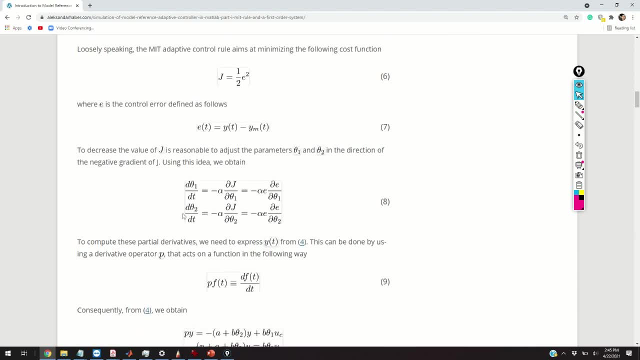 of the negative gradient of j. That is, we can simply state that the change of θ1 and change of θ2 in time should be in the negative direction of the gradient of the function j with respect to the parameters θ1 and θ2.. And now, if you compute these partial derivatives, 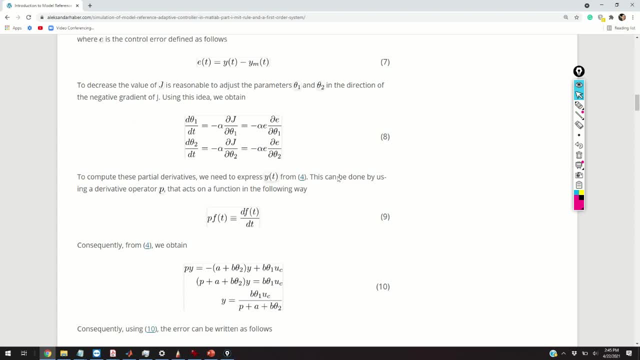 you will obtain the equation 8.. Now let us work around and let us try to find these partial derivatives To introduce the differential operator. this is a very important operator, So we can represent the derivatives as p times f of t. This is very similar to the Laplace approach, where 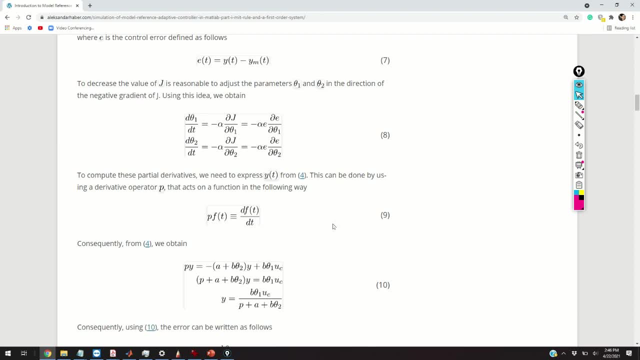 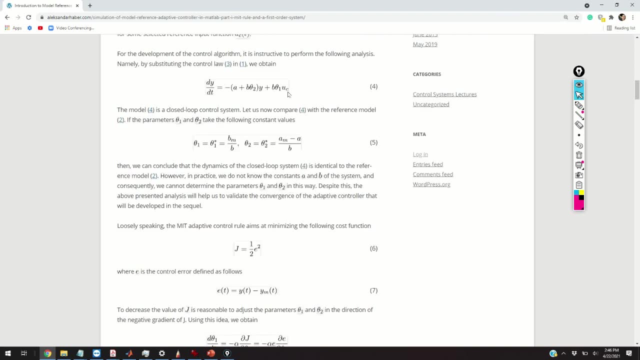 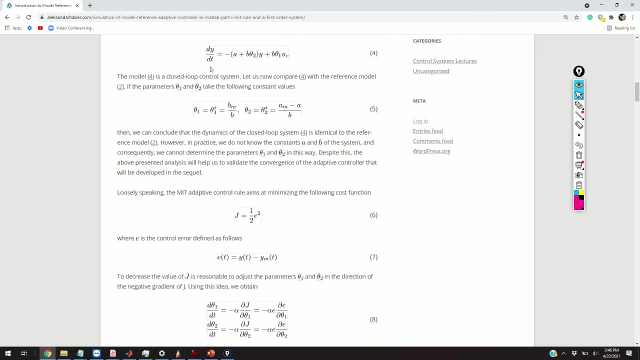 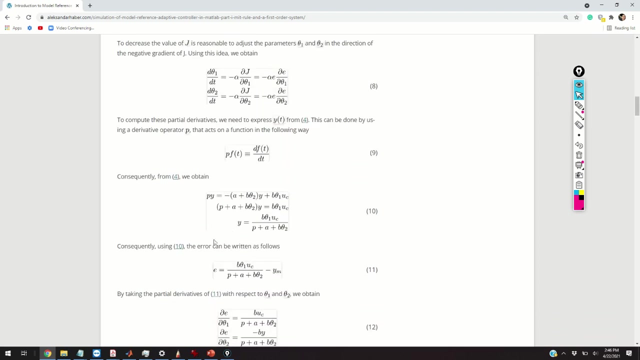 the complex variable s has an interpretation of taking the first derivative Consequently from equation 4, and equation 4,, if you look back, specifies our plan dynamics. we can simply represent this first derivative as p times f of t. We can just substitute the derivative as p times y right, And by working these expressions: 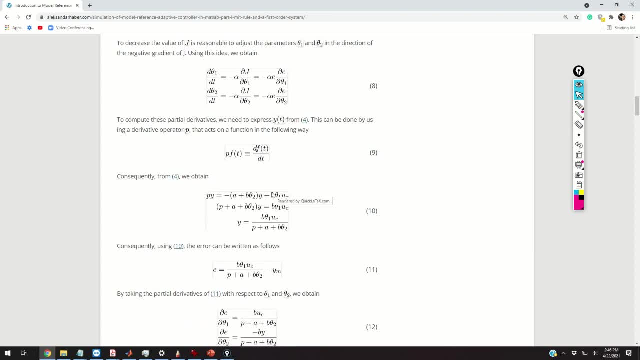 and a little bit doing massaging them. that's what we like to say in control engineering terms. we like to massage the equations. From this equation we obtain the output, And if we substitute this output of the plant into the system dynamics, we obtain the error. 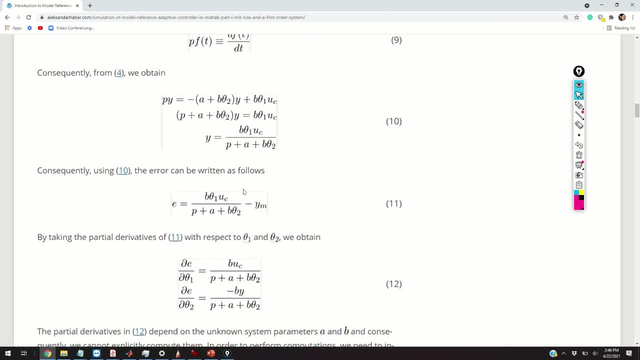 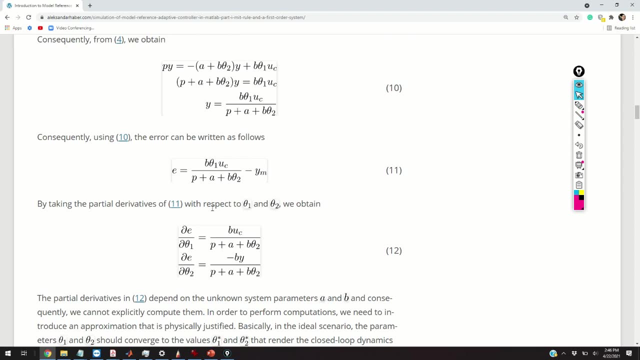 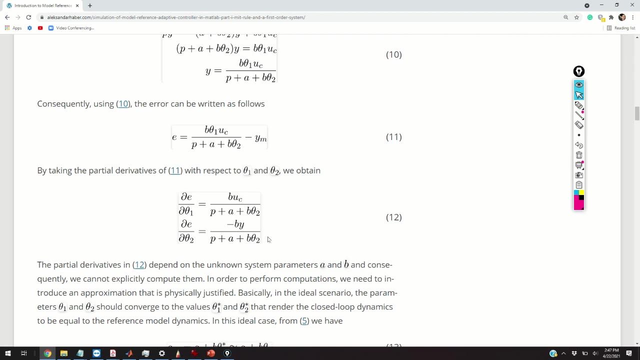 So the error is given by equation 11.. Now we can simply take the partial derivatives of e with respect to the parameters θ1 and θ2 and we obtain the expression 12.. So the expression 12 represents the partial derivatives. Now let us analyze these partial derivatives. Are they? 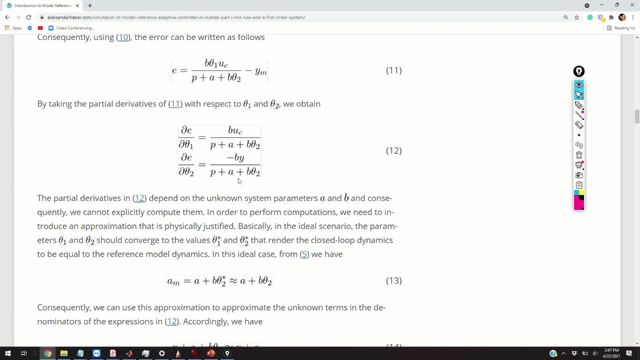 computable? Well, they are not, and the problem is that the parameter a and b are unknown, right? We don't know the plan dynamics, so we need to introduce some approximation Now. in ideal scenario, the parameters θ1 and θ2 should converge to the values θ1 star and θ2 star. 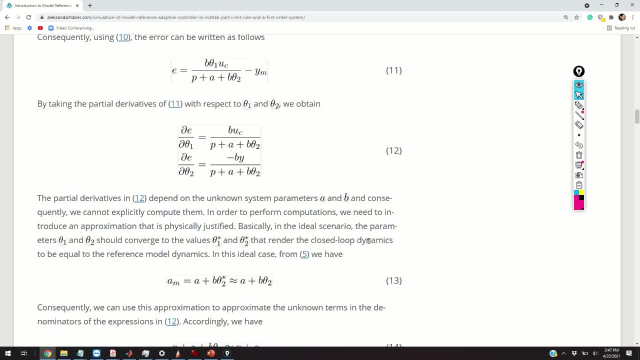 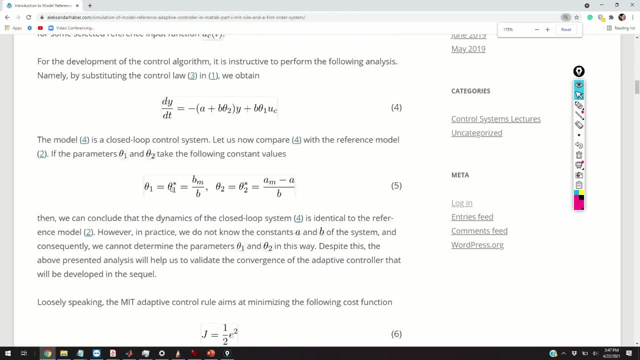 that render the closed loop dynamics to be equal to the reference model dynamics. Well, if you go back, so if θ1 is equal to θ1 star, bm over b and θ2 is equal to θ1 star, then we substitute the two parameters θ1 and θ2.. Now we have an. 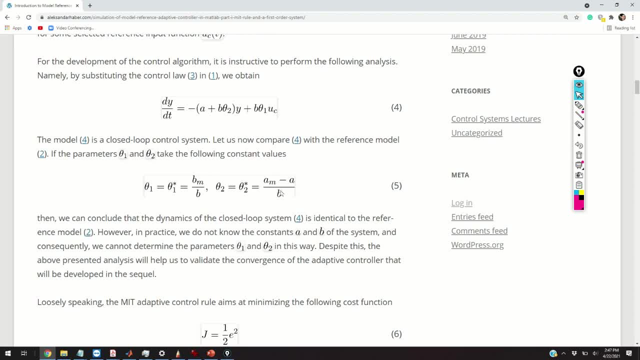 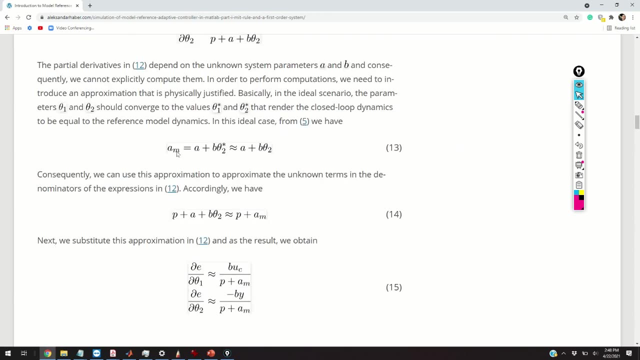 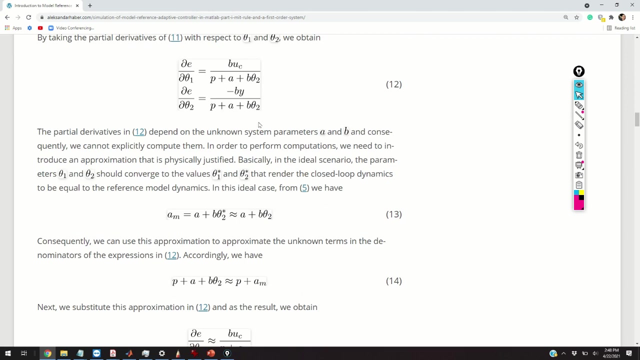 equal to theta 2 star, equal to am minus a over b, then we know that we have a perfect or the most optimal controller. well, from this equation, from the equation 5, we can use equation 5 to assume the following: we can assume that, basically, the parameters theta 2 are very close to the theta 2 star and this: 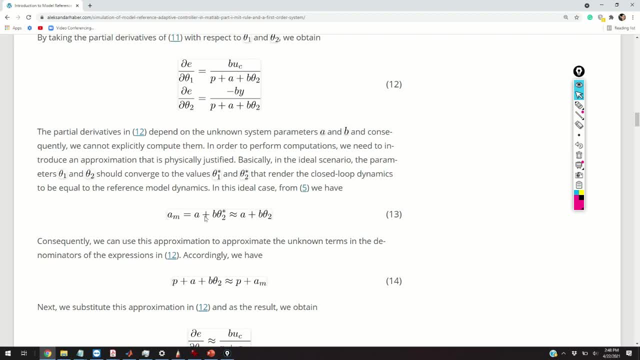 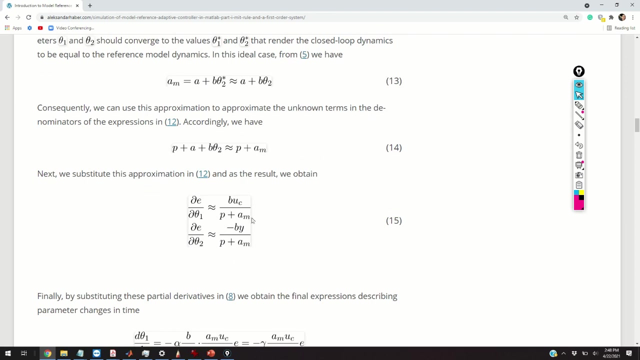 renders this whole term am to b for a plus p Norah to start, and this is approximately a plus batter right. and using this approximation we can approximate these 32 terms in the denominator and basically our partial derivatives become people, as am in the denominator right. so the de over the 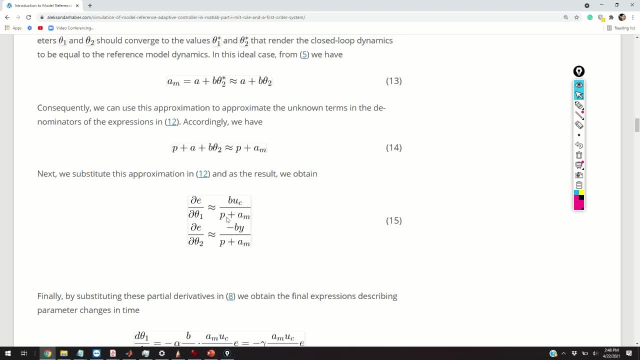 denominator power formula for the function of the unity of resultant two d, de is lifting. while she starts from the denominator over the Motan looking teta 1, theta 1 becomes BUC over P plus AM Now. but here is another problem: We still 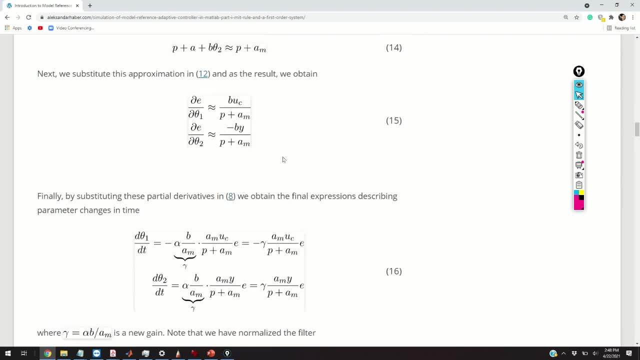 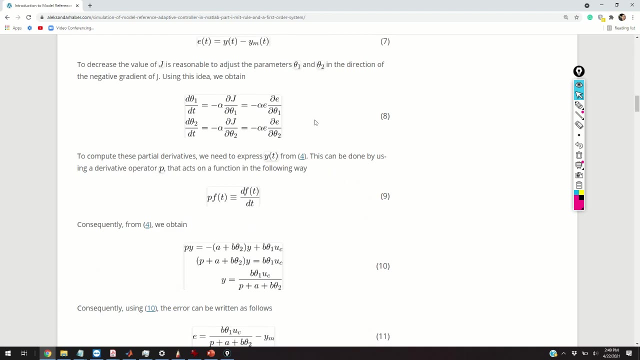 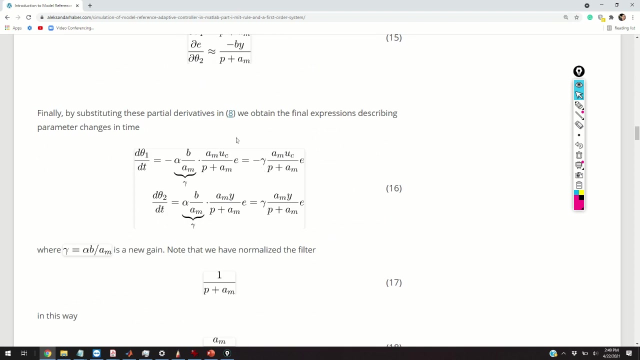 don't know B. Well, we can get rid of B. We can basically group it together with the control gain, And this is explained in equation 16.. Basically, by substituting the equation 15 in the equation 8, we obtain the equation 16.. Now, what can we do with this equation? 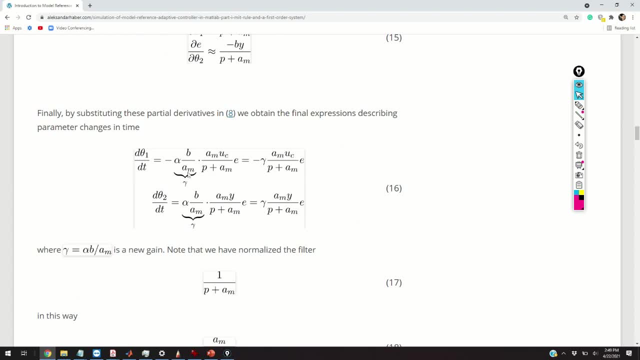 16?? Well, we can regroup the parameters and add additional parameters over here. Actually, we are not adding, We are just multiplying the equations by AM over AM. And what do we obtain? We obtain this term over here and this term over here, And now we can call this: 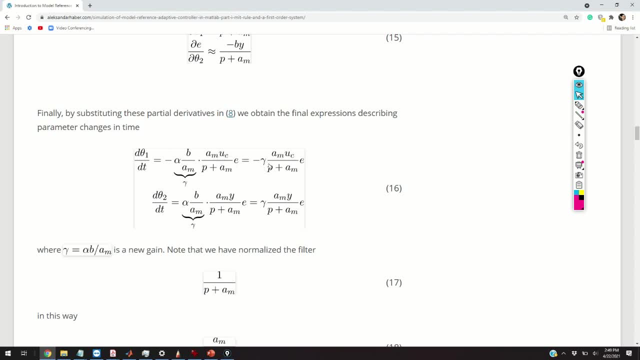 term gamma. This will be our control gain, That's adjustable parameter in the adaptive control algorithm, And final expression for theta 1 becomes: minus gamma AM times UC over P plus AM times error. Now everything here is computable if we specify gamma And we can freely choose gamma. You. 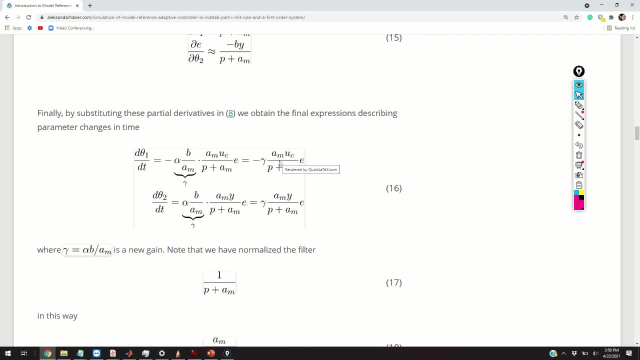 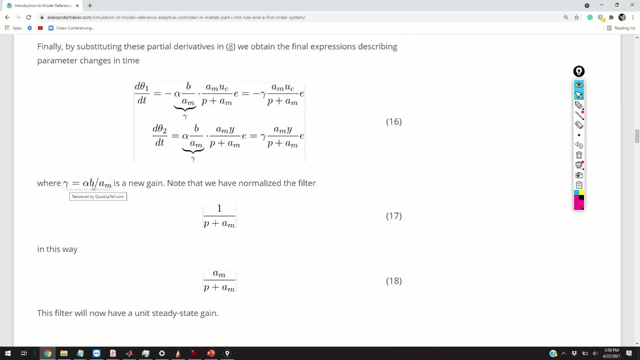 will see later on in MATLAB simulations how to. how does the parameter gamma influence the system dynamically? We do the similar trick with d, theta 2 over dt, and we obtain the final expression given by this equation. And, as I said previously, alpha times B over AM is a new control gain. Now one important. 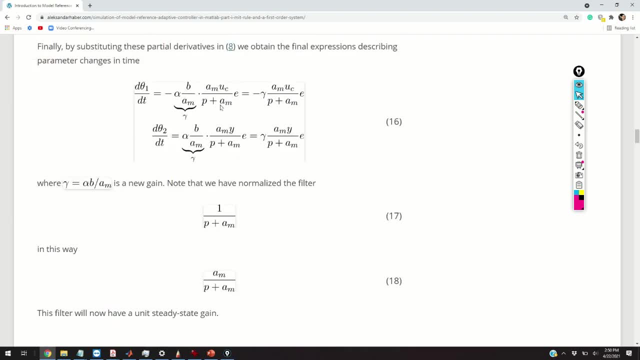 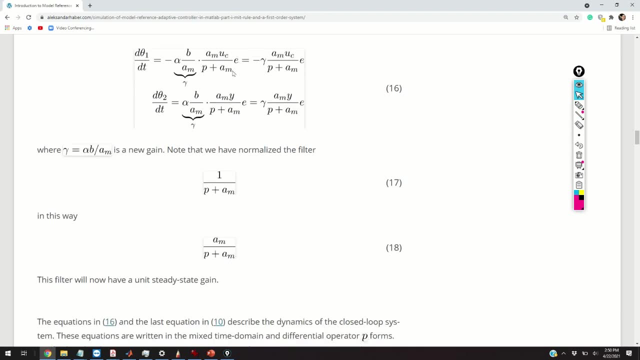 thing has to be mentioned here: we have normalized the control gains. We have normalized the control gains in this way, basically- or actually not the control gain- we have normalized this filter 1 over p plus am and it becomes am over p plus am. In this way we achieve a steady state gain of 1. 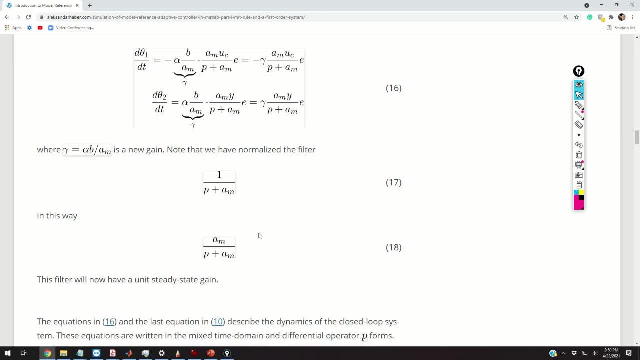 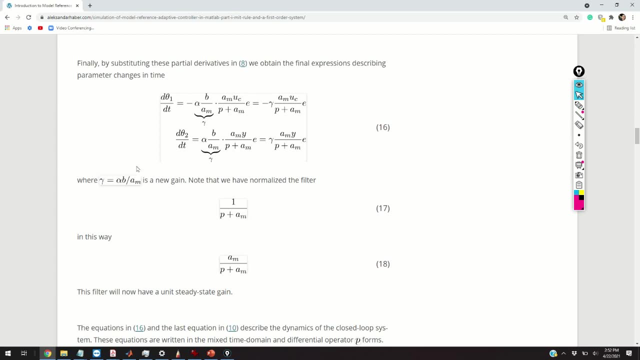 which is very convenient for a control algorithm. The equation 16 is very important since it specifies the change of the parameters theta 1 and theta 2 with respect to time. We see that theta 1 and theta 2 are the functions of error, control, gain, system output and the input to the reference. 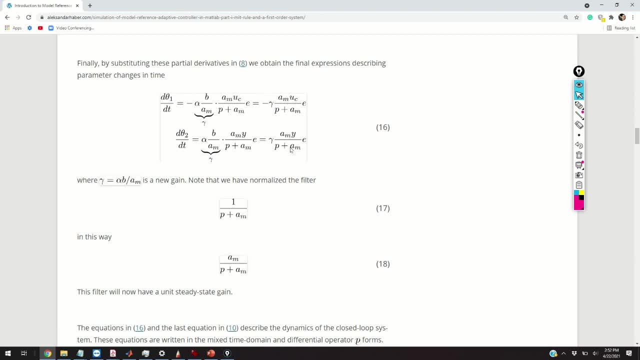 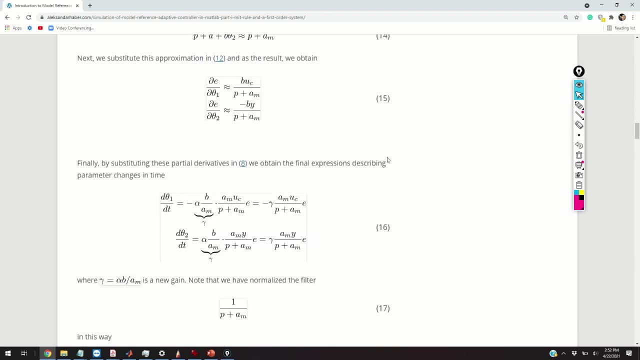 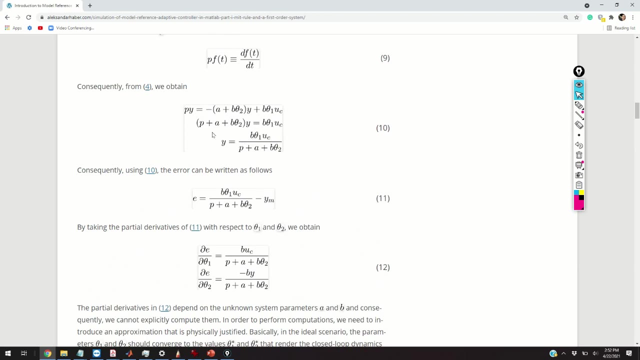 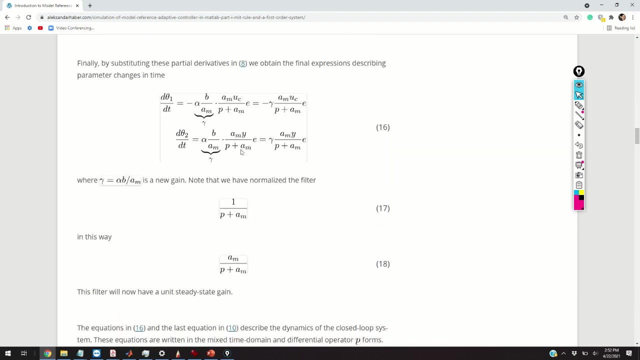 model and plus we have these filters over here. These equations in the equation 16 should be coupled with equation 10.. The equation 10, its form over here- describes the plan's dynamics. So equation 16 and 10 specify the dynamics of the closed loop systems. These equations are written in: 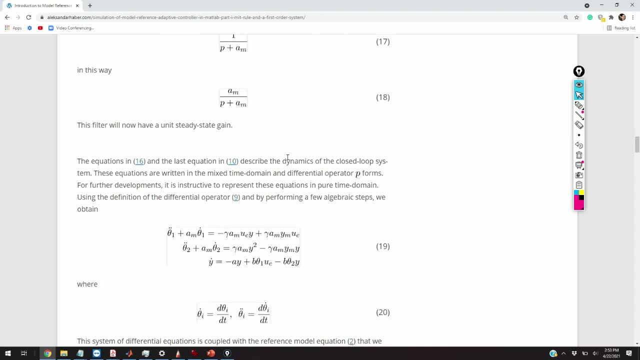 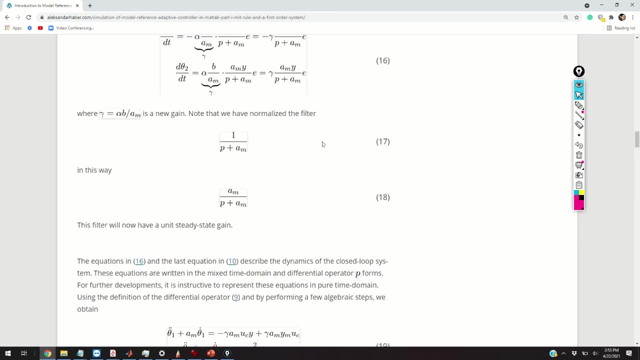 the mixed time domain and differential operator P forms. So in order to simulate these two equations, we need to convert them to pure time domain and we need to write a states-based model. So after a few algebraic steps, mainly we want to get rid of these P differential. 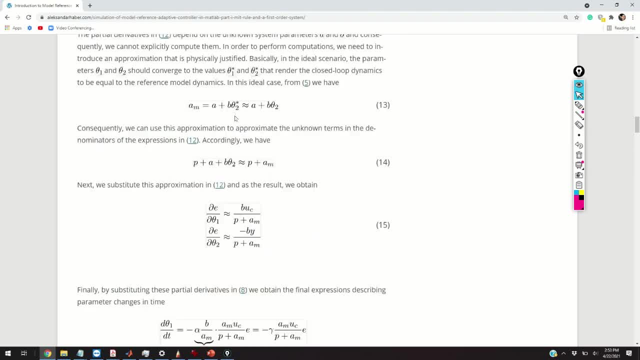 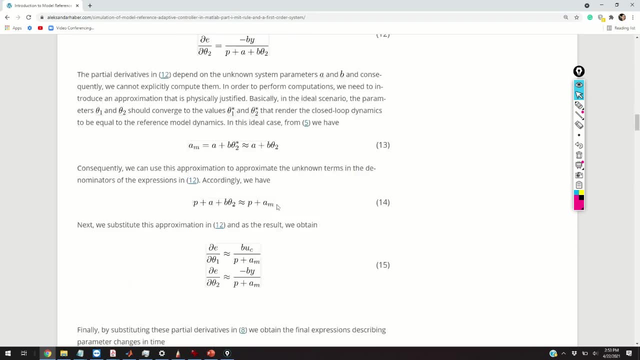 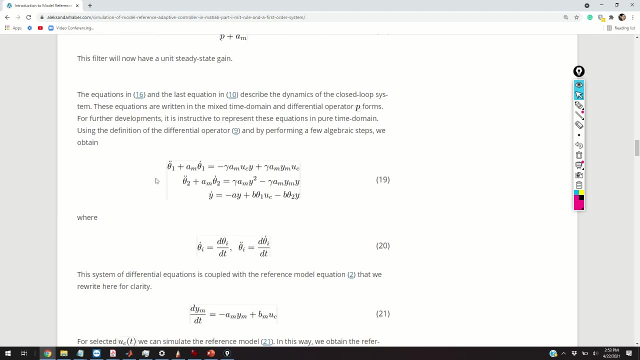 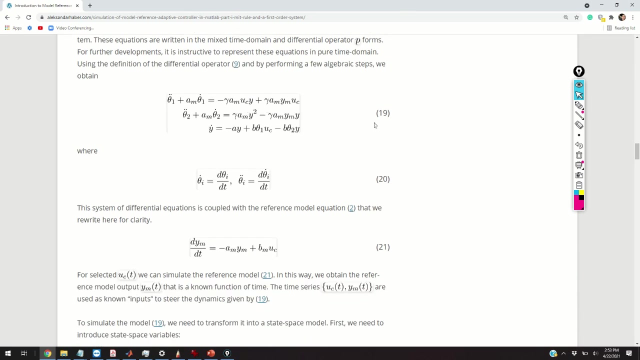 operators here and here and here, and the equation 10. we can simply do that by revoking the definition of differential operator and at the end we will obtain the state space model. actually, it's not a state space model. this is still a system of three differential equation and we need to write these differential equations in. 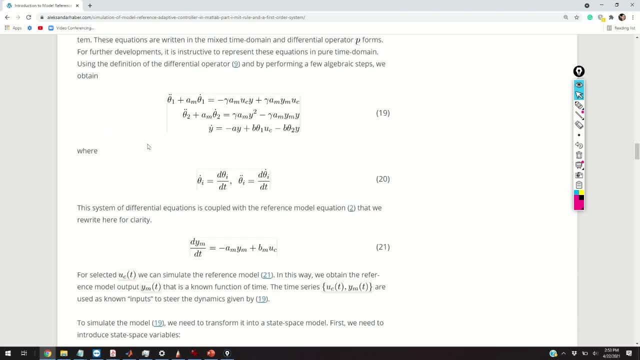 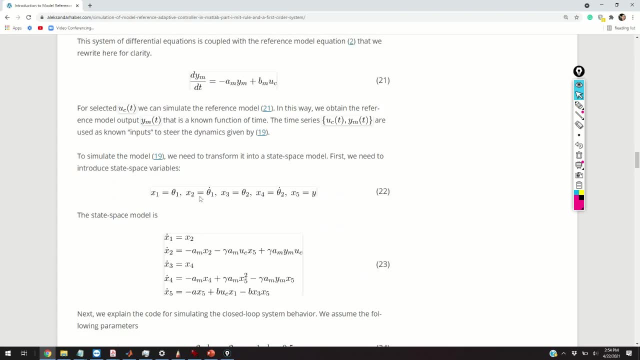 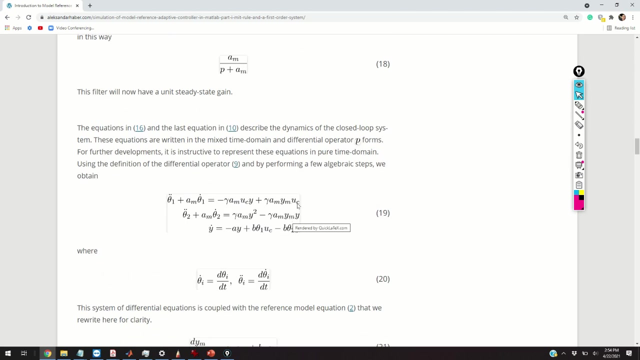 state space form. how to do that? well, we can simply introduce the state space variables: x1 is theta 1, x2 is theta 1 dot, x3 is theta 2, x4 is theta 2 dot and x5 is the output y. now you might ask me: how about ym, ym and uc? what happens with? 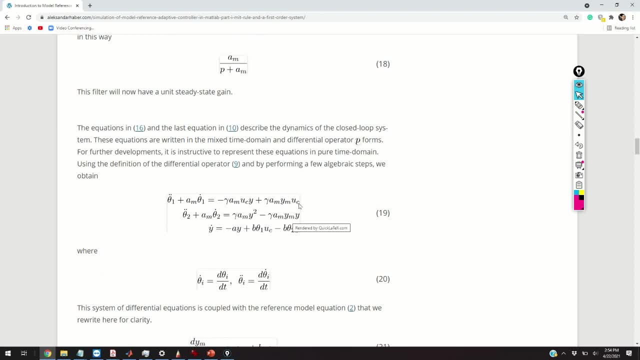 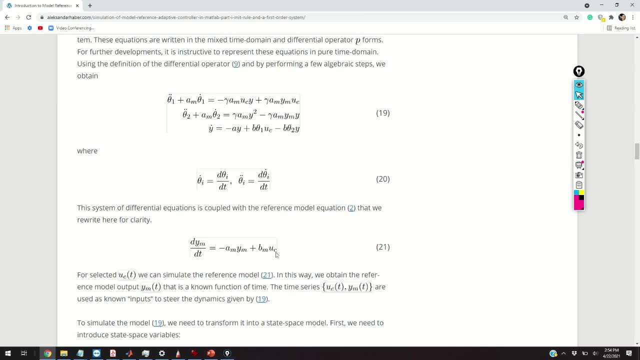 these variables? well, these variables are known functions of time, because we can simulate the state space model in a state space form and we can simply calculate the dynamics of a reference model for for known value of uc and we can obtain ym. so they act as inputs, they drive this model. they drive this model. 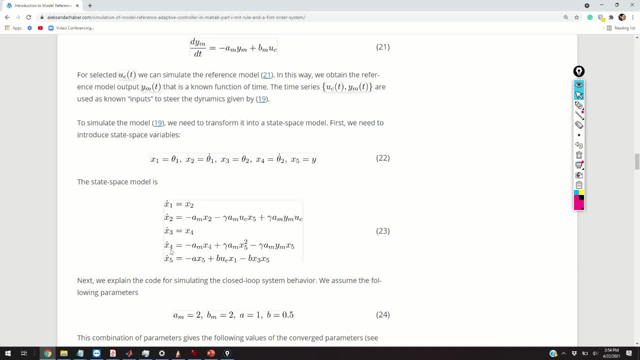 so at the end you can see over here that our original system that was of first order, becomes a fifth-order state space model when we couple it with adaptive controller. so this is actually a model called phase space model and we can. So this is the price that we need to pay for an adaptive controller to increase the system order. 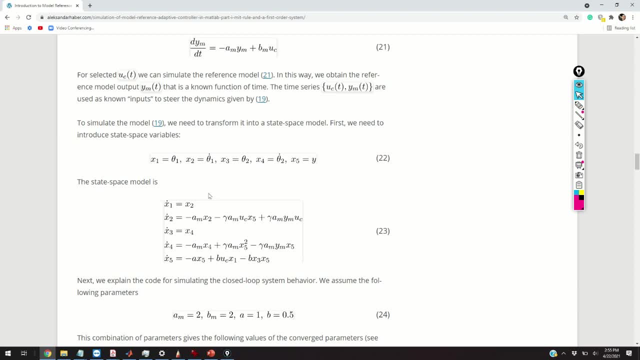 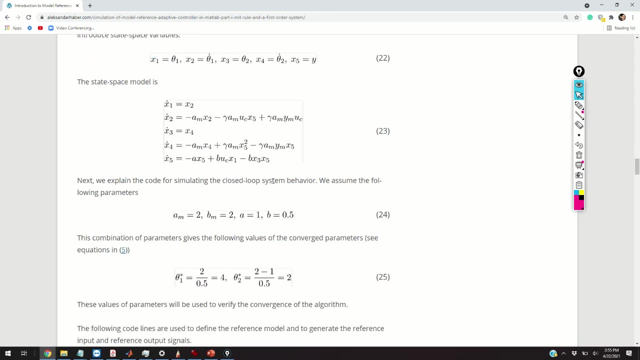 And, moreover, you can observe that this is a non-linear states-based model. right, Although the dynamics is linear, when we couple dynamics with the adaptive controller, the system becomes non-linear. That's why you should study non-linear control systems. Okay, so this is our states-based model. 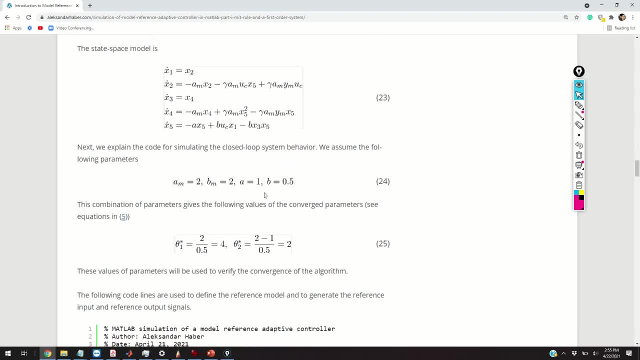 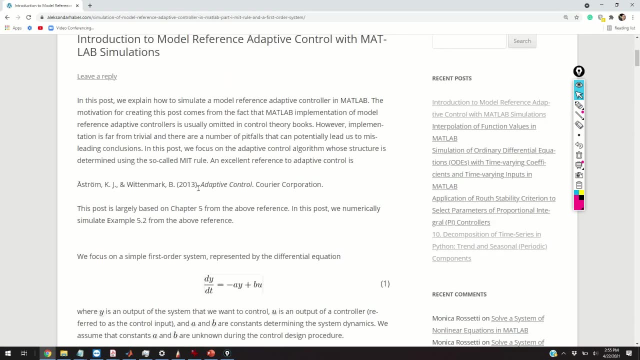 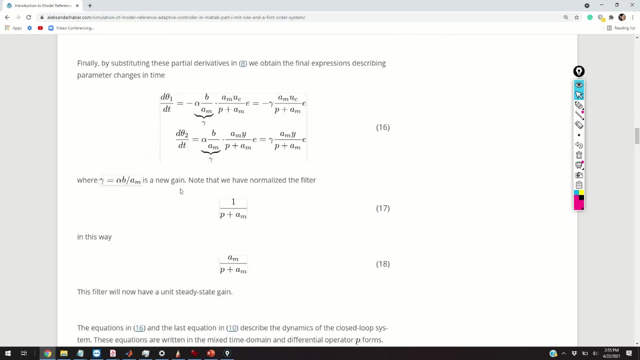 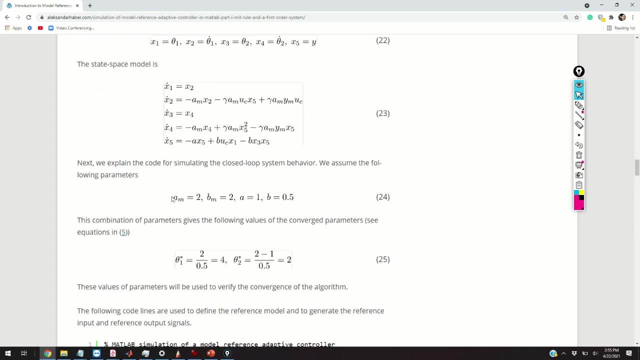 And let us simulate its behavior. So I'm just taking one of the examples from this book, from a famous reference on adaptive control by these two very well-known authors, And the example number is 5.2.. So I'm taking the 5.2 example, I'm taking the same variables and I'm simulating the system dynamics. 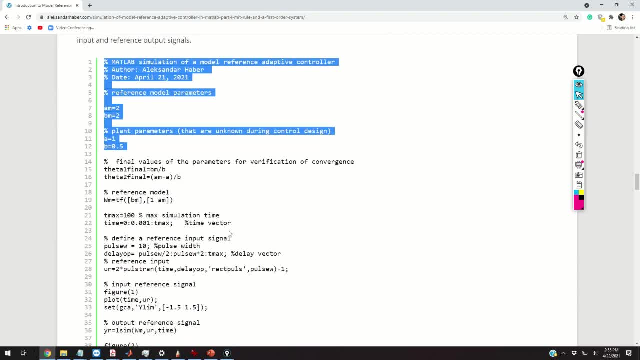 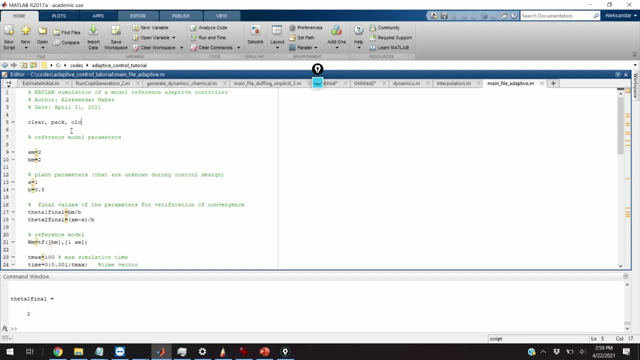 And so here is the MATLAB code for simulating the system dynamics And in the SQL, I will explain. Before I start, I have to mention that all the codes in this video will be posted on my GitHub page. A link to my GitHub page is given in the description below. 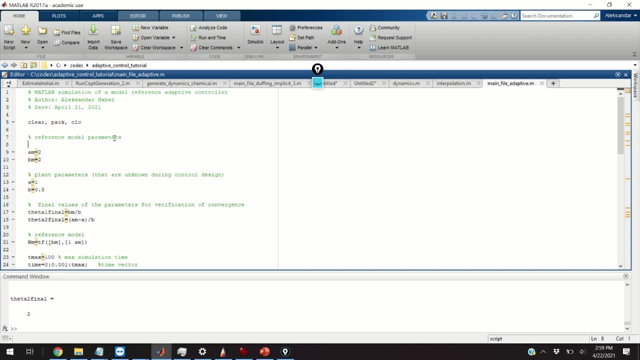 So let's start. First we need to specify the reference model, parameters, the planned parameters, And we can simply compute the final values of the parameters for verification of the convergence. Then we specify the reference model by simply typing a transfer function: bm in the numerator and 1 plus am in the denominator. 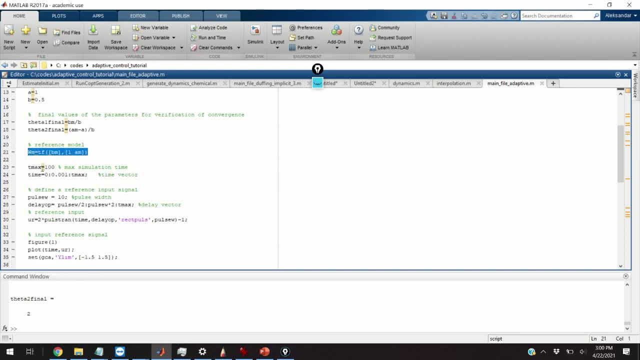 So this is our planned right. Then we specify the maximum or the maximal simulation time, We specify the time vector And we define a reference input time And we specify the input signal, which in our case will be a pulse signal. 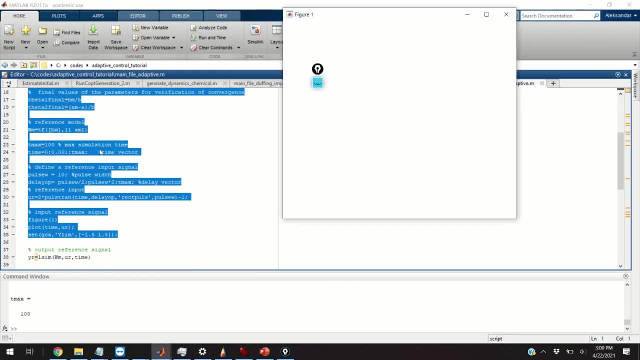 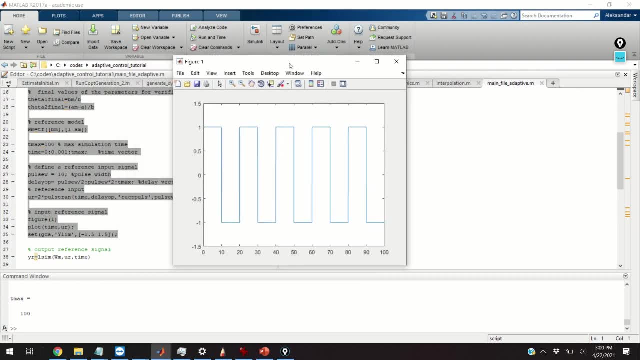 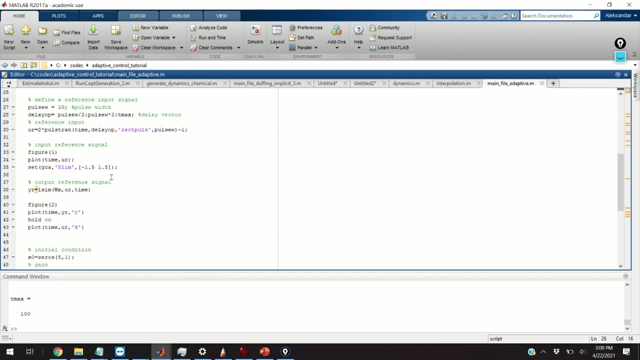 So let's see how does our input signal look like. So this is our input signal. This is an input to the reference model, And let us simulate the reference model or our desired system for this input. And let us simulate the reference model or our desired system for this input. 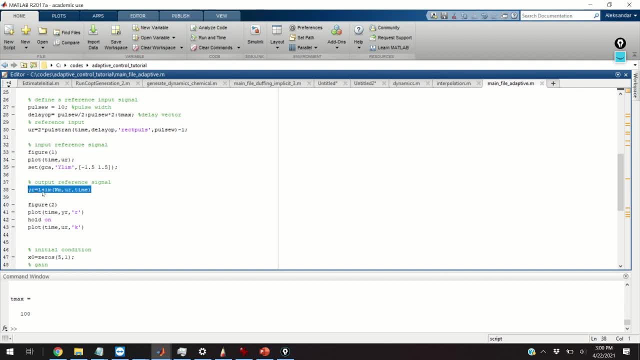 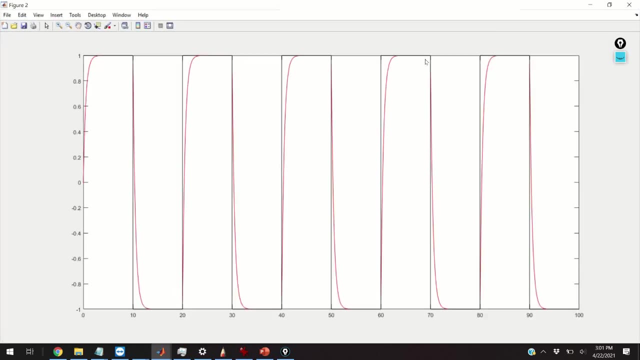 We can do that by simply using the MATLAB function lsim. We specify the transfer function, We specify the input And we specify time vector. Let's see what happens. Okay, So let us analyze the results. This red line is the output of the reference model. 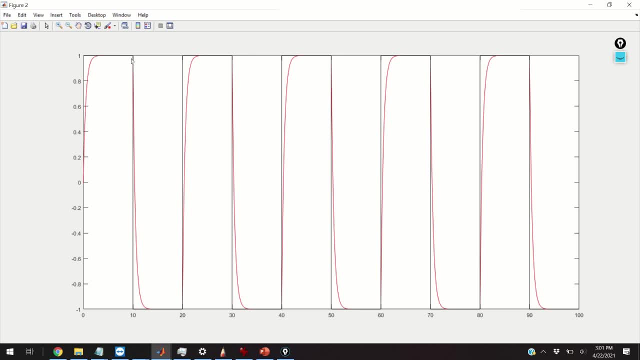 And the blue line, or actually the black line, is the input to the reference model. that is again red line, the output of the reference model and the dark or the black line is the driving input. we can see that after some transients the output follows the input. 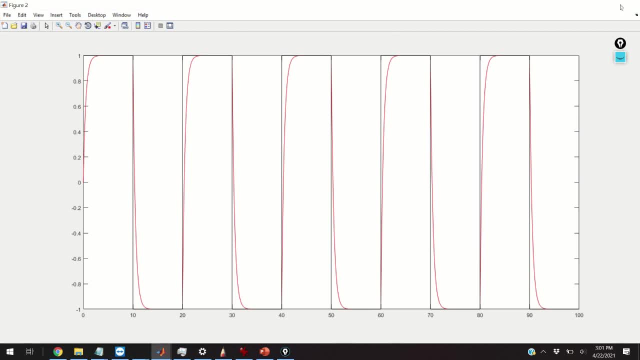 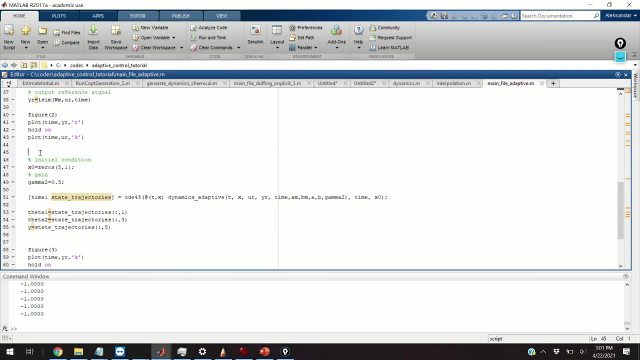 this is because the system is stable, okay, so let's continue. the next step is, of course, to simulate system dynamics, the closed-loop system dynamics, and to simulate the adaptive controller. to do so, we need to specify, basically, the function that defines the closed-loop dynamics. so I'm going to open this function. 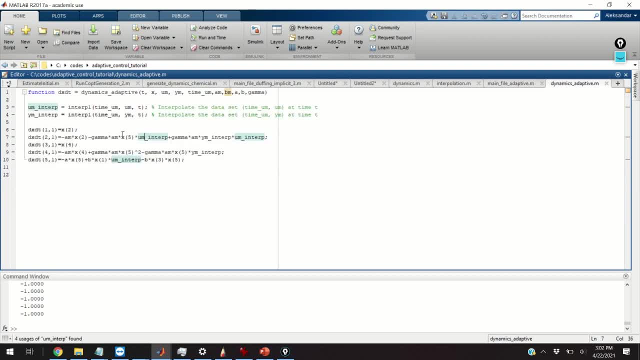 here's our function. it's called dynamics adaptive. this function takes time and x as inputs. t is a scalar, x is a five times one vector. um is the vector representing the time series of the reference model. inputs, ym is a vector representing time series of the output of the reference model. so these two variables. 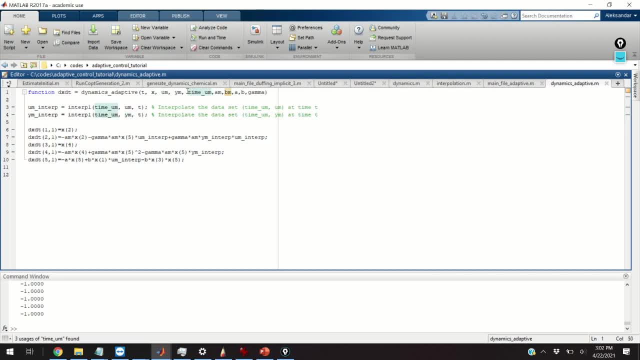 are known and act as inputs. this is the time vector for simulation. am, bm, a and b are actually parameters and gamma is the control gain. now here's the trick. so, since OD45 cannot accept time-varying inputs or time-varying parameters, 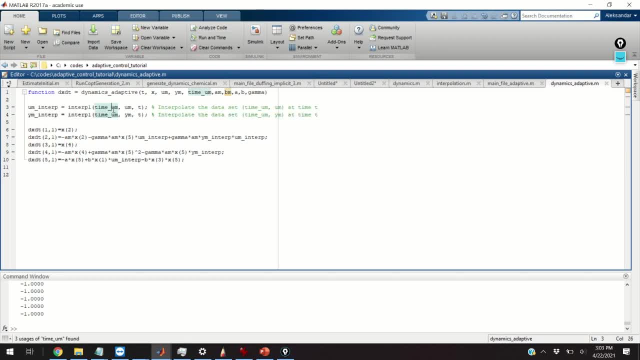 we need to do the following trick. so we're going to interpolate from um and from ym the values specified at certain times t, so we're going to use this trick. i have created a complete video that explains how to do that, and you can read more about this video and this approach. 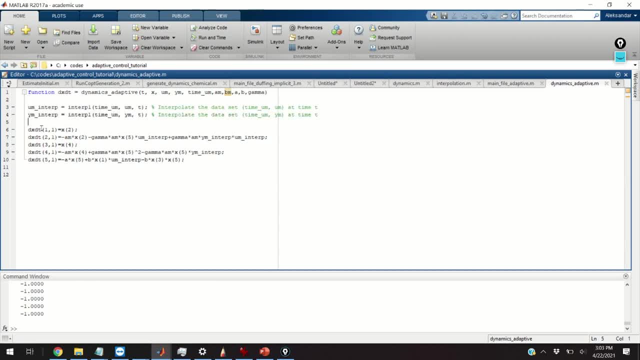 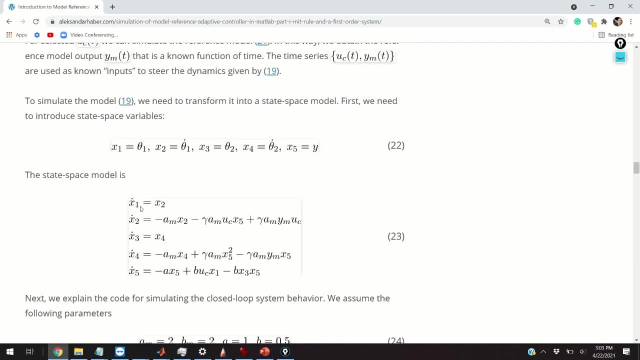 in the post that I've previously explained and here's our dynamics. so this is the dynamics of our system and if you go back here, so these are the state-based variables and let us compare. so x1 dot is equal to x2, x1 dot is equal to x2. 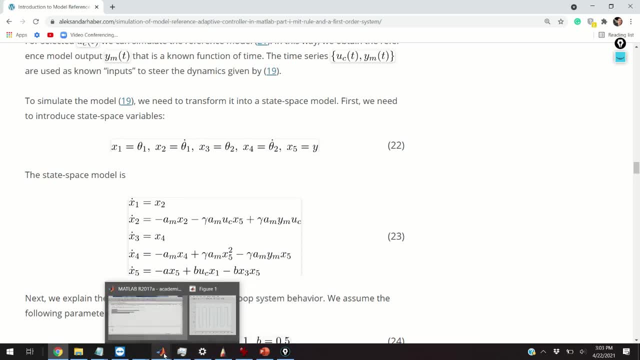 x2 dot is equal to x2, x2 dot is equal to x2, x2 dot is equal to x2. So let us go back to our code and we can see here: dx, dt 1,, 1, is x2.. 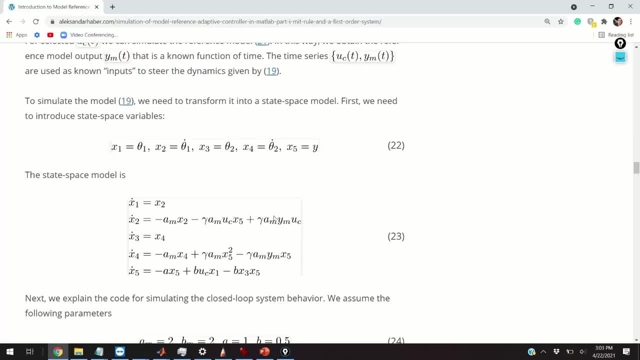 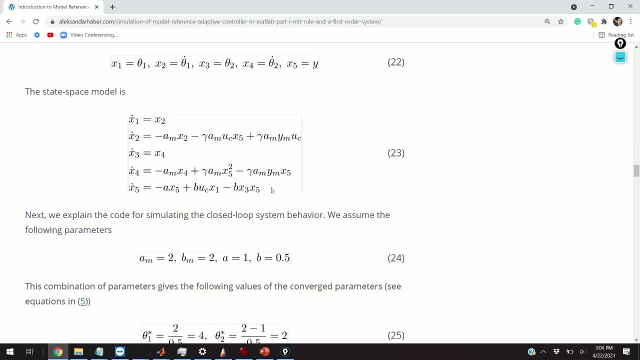 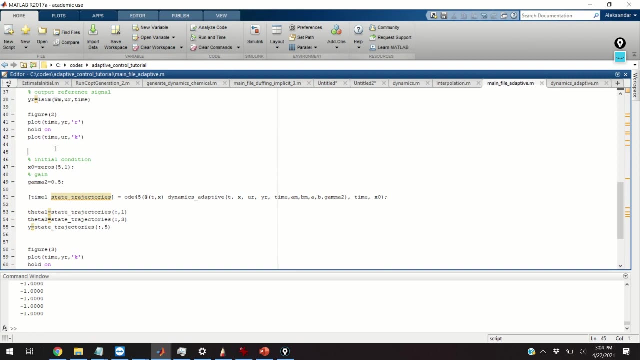 This is the first equation, This is the second equation, the equation over here, etc. Third, fourth and this is the fifth equation that you can see over here Now. we are basically now ready to simulate the system dynamics. So first we specify the initial condition: zeros. 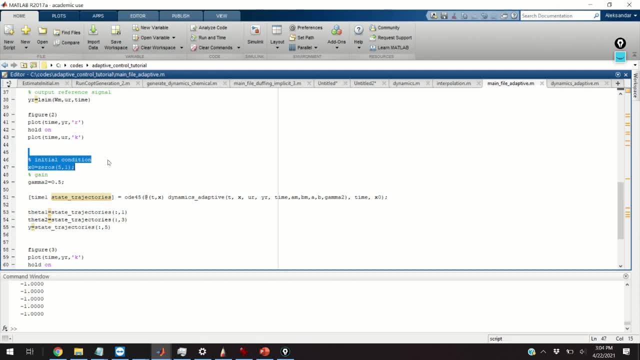 Although you can also specify arbitrary system conditions and you can specify the gain gamma. In our case, we are going to select gamma 0.5, and we want to see how does the system behave for this parameter: gamma 2, equal to 0.5. 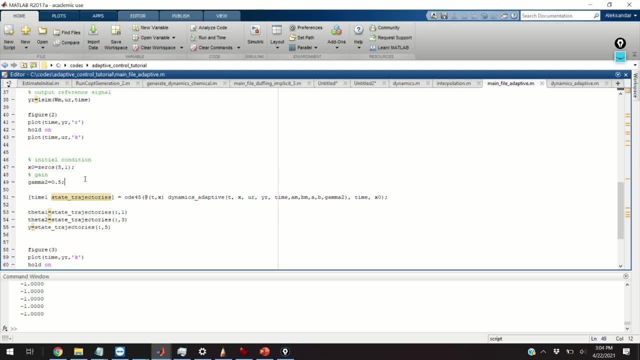 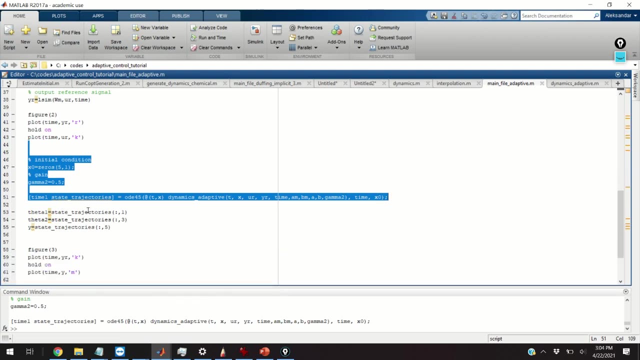 You can change it to any value You might obtain. maybe unstable behavior, watch out. So let us do that. So we simulate the system dynamics. It is going to take a while. Although I am having a new computer, we are still. we still need few seconds to simulate the system behavior. 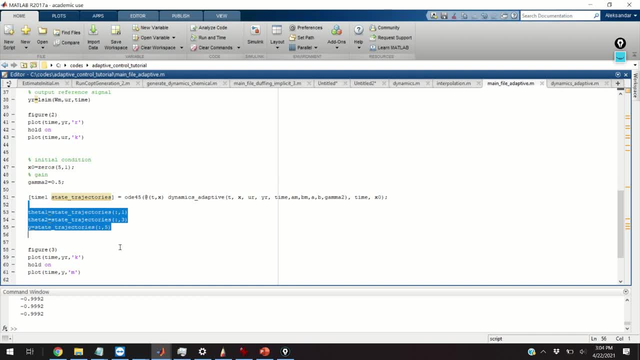 And let us extract the state space variables, because the state trajectories, the output of this simulation, contains a matrix, basically, that has five columns And the number of rows is equal to the number of samples. So this is actually the way that five homemology elements manipulate the system. 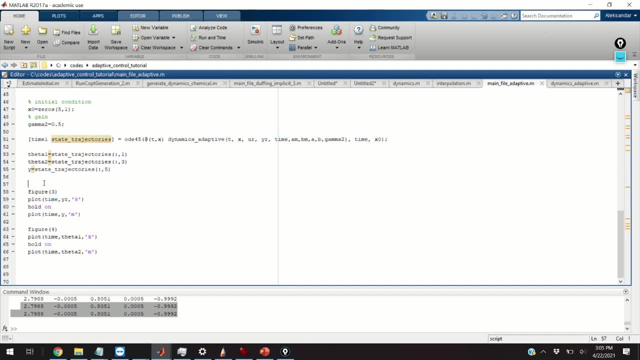 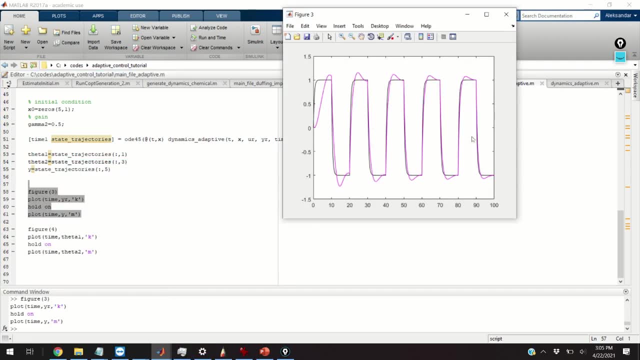 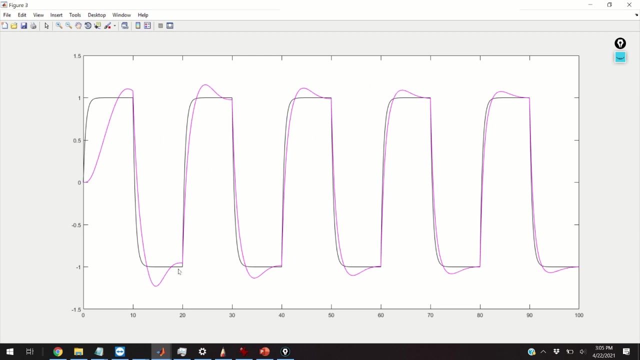 So we will� Taiwan vector And let us plot the system response. So first we are going to plot the output of our reference model and the output of our plant. The purple line is the output of our plant and the dark line or the black line, which is the output of the reference model. 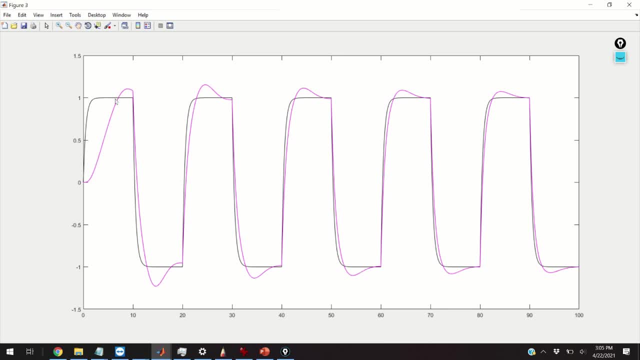 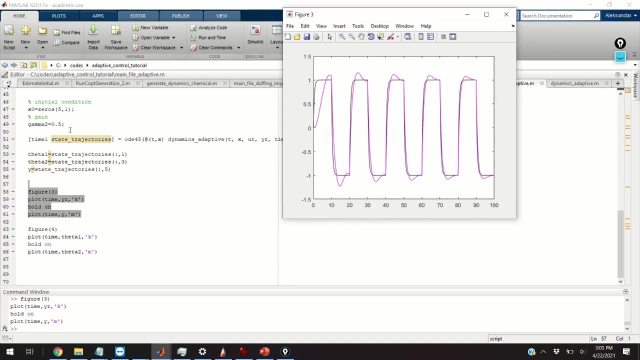 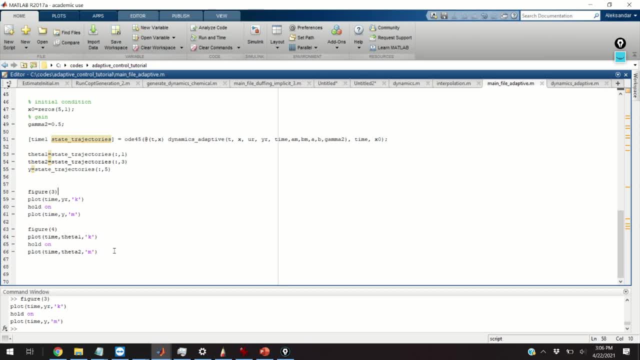 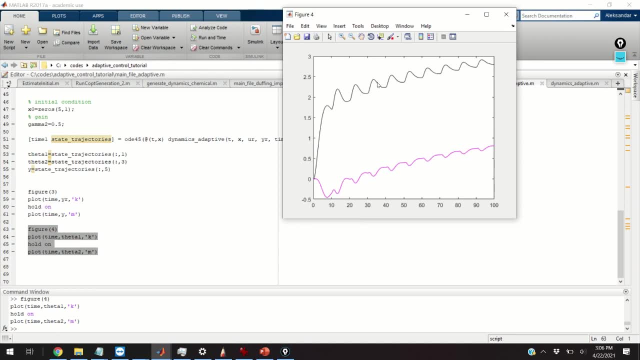 increase this parameter to obtain a better tracking performance. and finally, we can plot the trajectories of the parameters theta1 and theta2.. The dark line, the black line is theta2 and basically the purple line is parameter theta1 and the desired values are basically not desired, the most optimal. 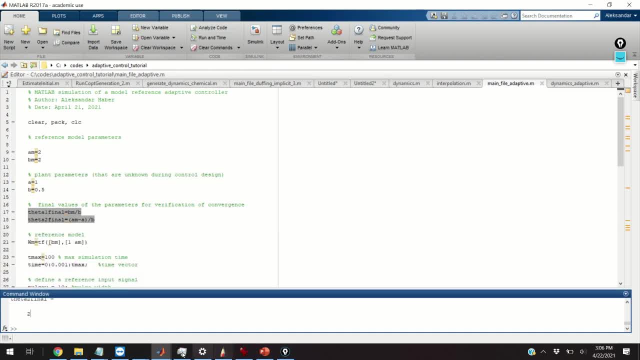 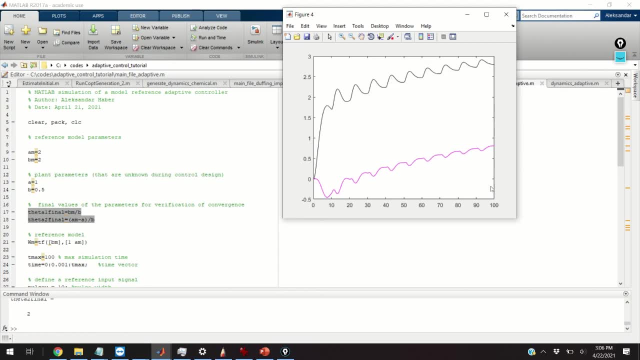 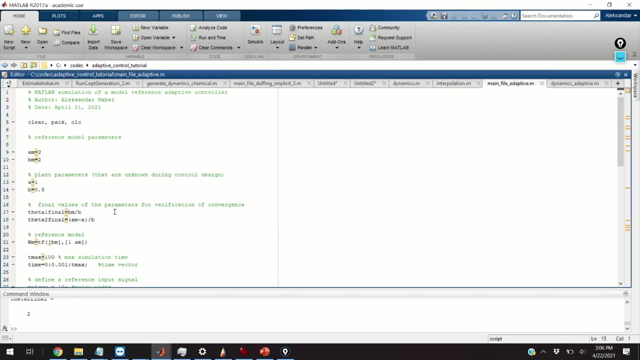 values are basically 4 and 2 and by observing these transients we see that basically theta1 and theta2 are kind of approaching these parameters. We didn't simulate the dynamics for more than 100 seconds. however, we can do that and you can observe that these parameters will. 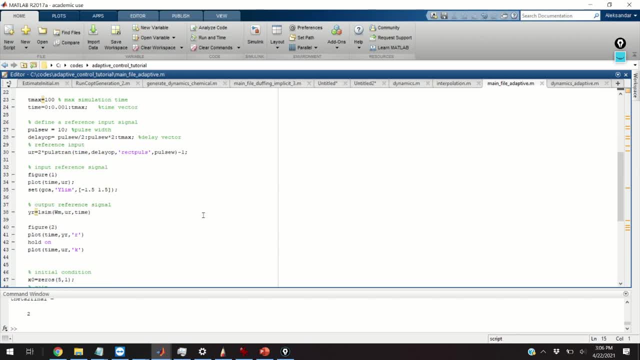 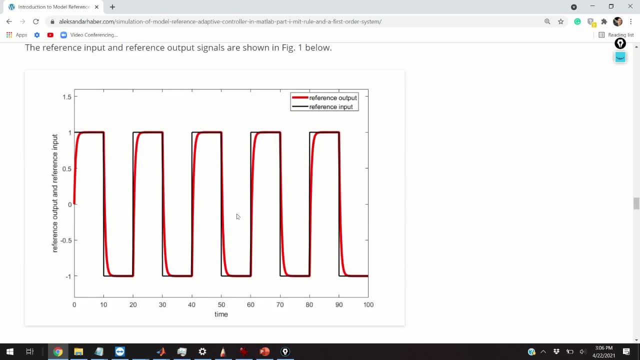 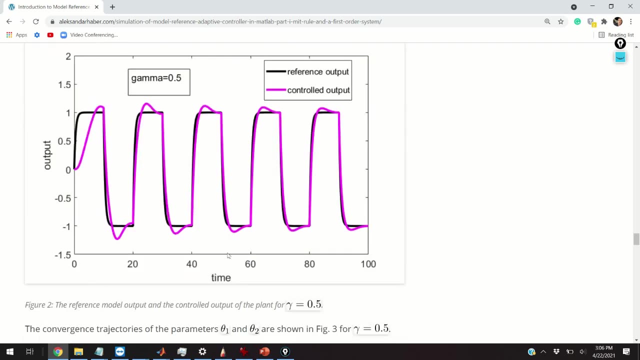 converge to the most optimal values. So let's see what happens when we increase the parameter values, and I'm going to go back to the post, since I've generated the simulation results. This is the first graph you have seen, right? This is the second one. This is basically the 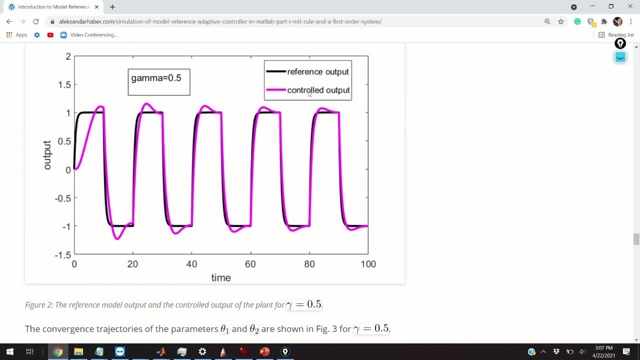 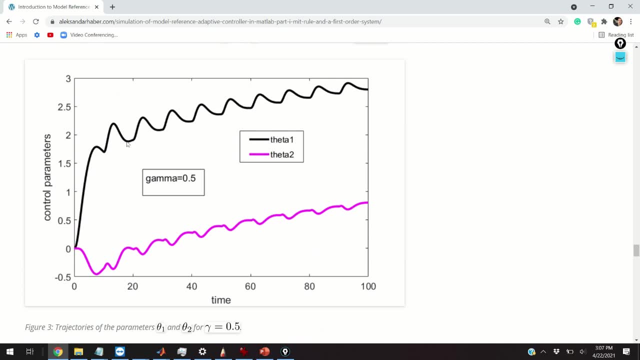 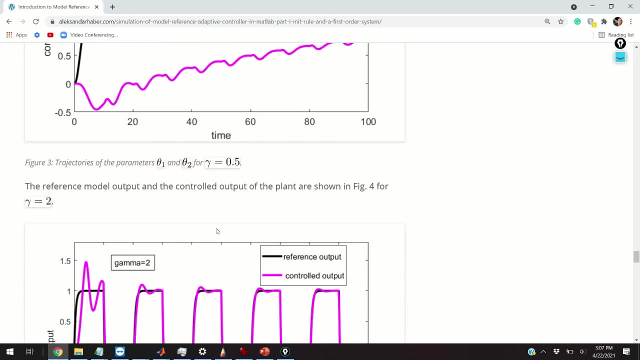 comparison of the reference output and the controlled output of the plan for gamma equal to 0.5, and this is the parameter convergence for, basically, theta for gamma 0.5.. You can see theta1 and theta2.. Okay, so let's see what happens when we 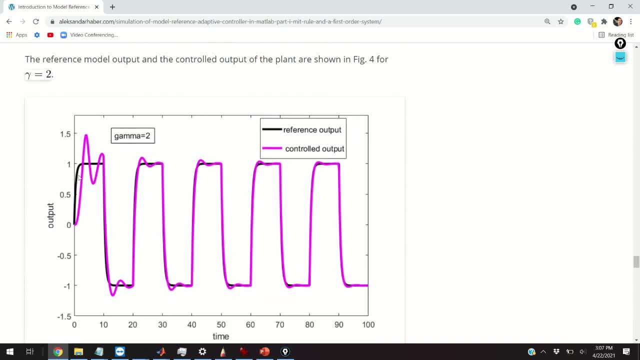 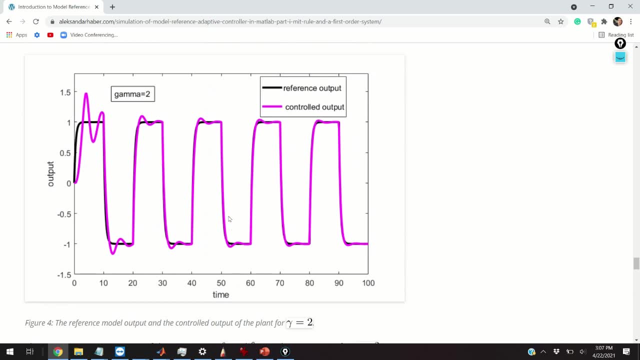 increase gamma to 2.. Well, we see a dramatic change. First of all, we can observe that the tracking performance after, let's say, 50 seconds is almost perfect. However, the price we need to pay is, basically, is increase in. 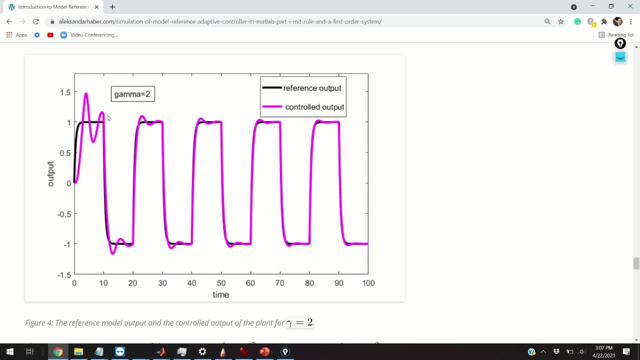 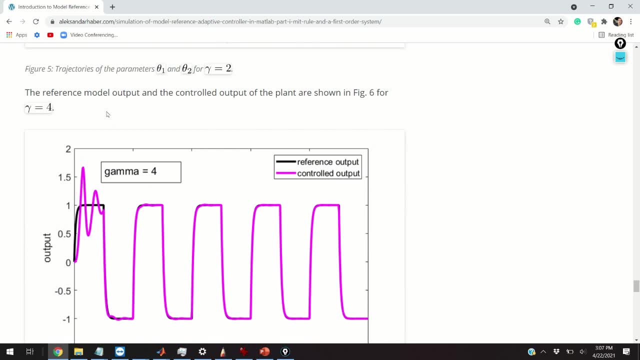 overshoot right. We see more overshoots over here. Now let us try to be more aggressive and let's try to basically increase gamma to 4, and this is what happens when gamma is increased to 4.. So the figure 6 represents the case when